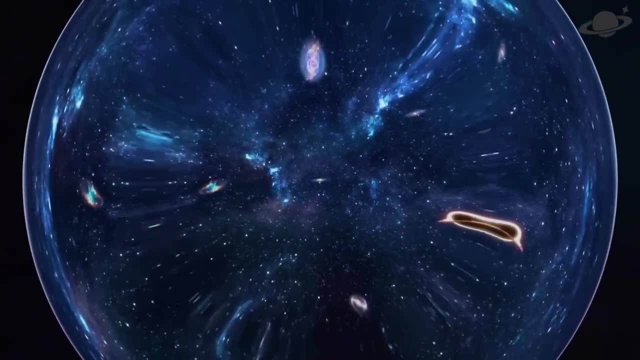 expands, driven by the enigmatic force of dynamism, the universe will become more and more dark. As the universe expands, driven by the enigmatic force of dynamism, the universe will become more and more dark. It gradually cools down as its energy disperses across a growing volume. Eventually, all stars will exhaust their nuclear fuel, fading into darkness. Galaxies will drift apart and, over immense timescales, black holes will evaporate. In the distant future, the universe will reach a state of maximum entropy where there's no significant energy exchange, rendering it uniformly cold and dark. 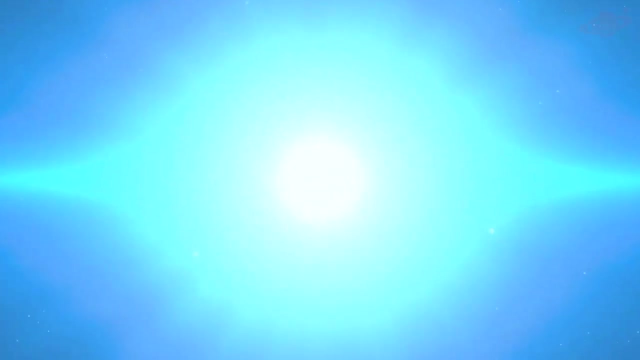 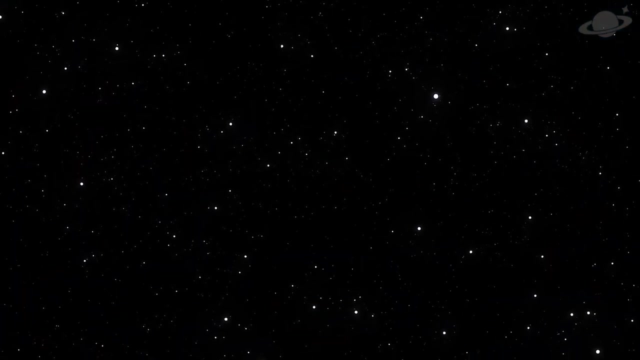 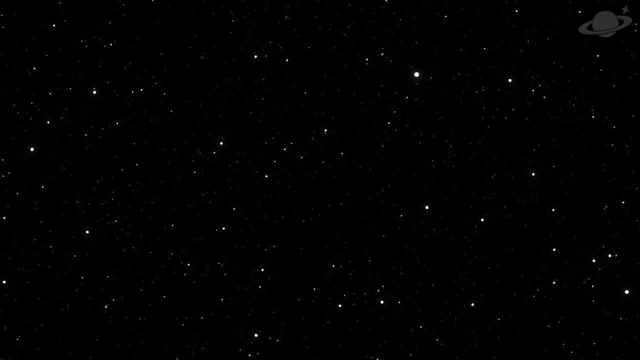 This Big Freeze scenario is the most probable outcome according to our current understanding of cosmology, particularly based on measurements of cosmic microwave background radiation, the lingering light from the Big Bang and observations of the universe's accelerating expansion. These observations suggest that the universe is flat and will likely keep expanding. 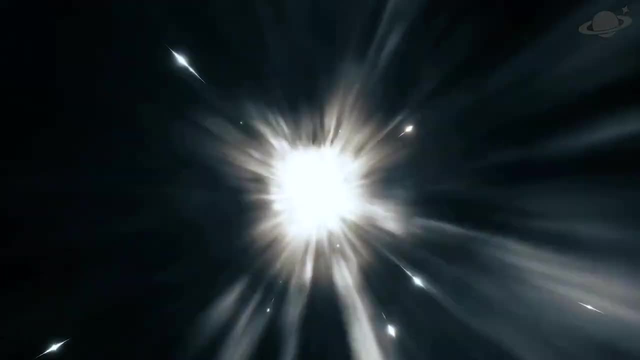 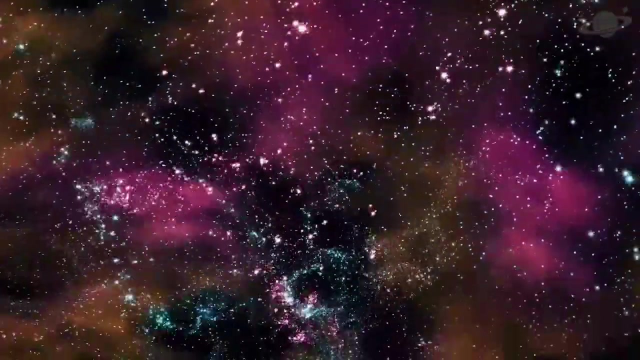 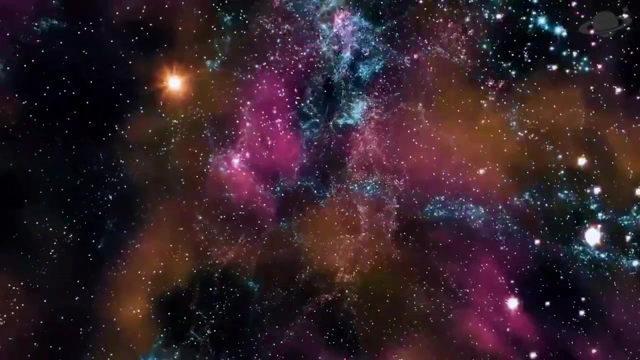 indefinitely. While this paints a bleak picture of the universe's far future, it's important to note that this isn't something imminent, but rather something that will unfold over an incredibly vast span of time beyond our grasp. We're talking about timescales in the trillions of years far surpassing the universe's current age. 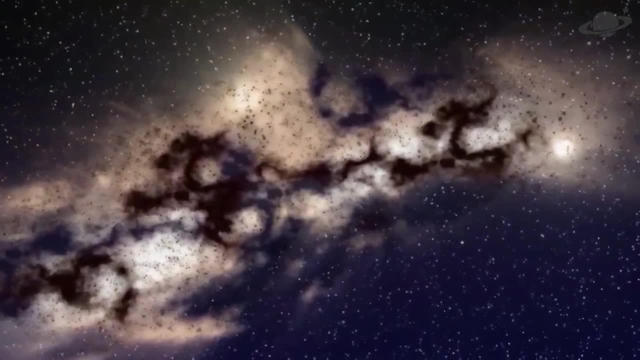 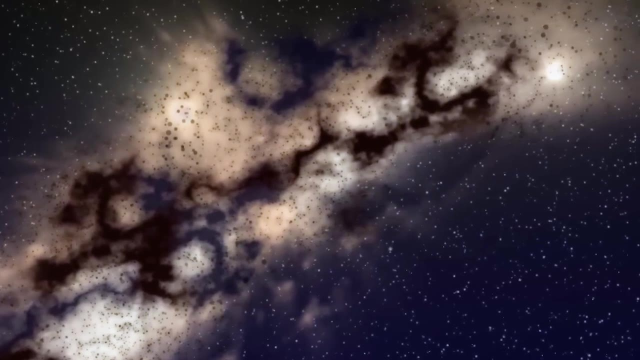 of about 13.8 billion years. Our understanding of the universe's fate has evolved significantly over the years, thanks to advancements in technology, astrophysics and theoretical models. This journey began in the early 20th century, with astronomers like Edwin Hubble. 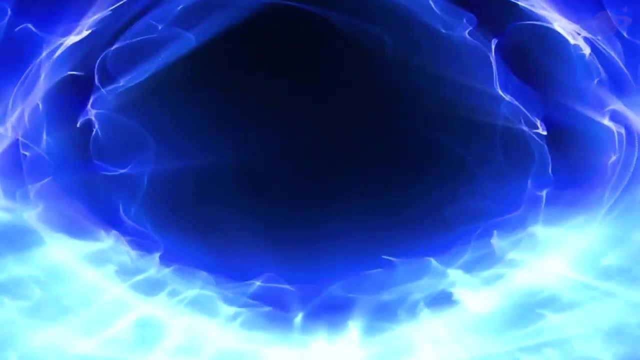 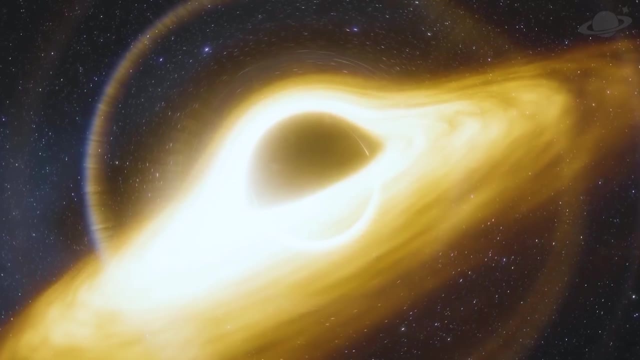 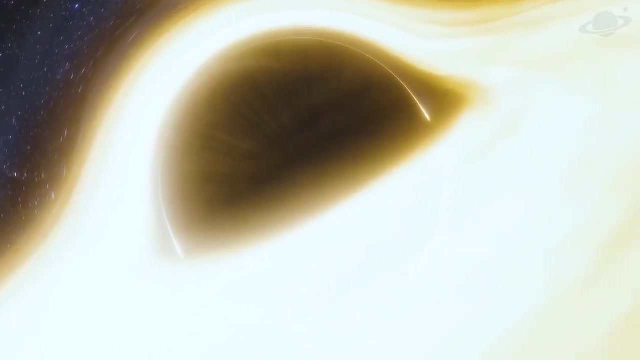 whose observation of the redshift in light from distant galaxies provided the first solid evidence of the universe's expansion. This discovery was pivotal, shifting scientific consensus away from the belief in a static universe. In the following decades, scientists wrestled with the implications of this expanding universe. Early models suggested that if the 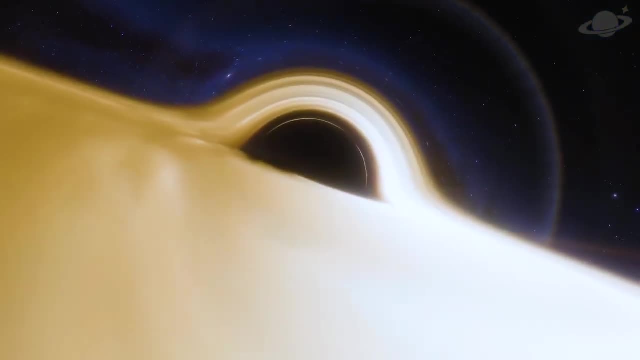 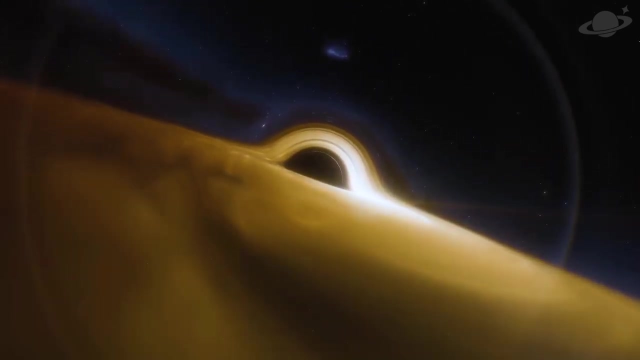 gravitational pull of all matter was strong enough, it might eventually halt expansion and lead to a Big Crunch where the universe collapses back in on itself. This theory suggests that the universe is not a big crunch but a big crunch. Another theory suggested a cyclic view of the universe, where each collapse or crunch 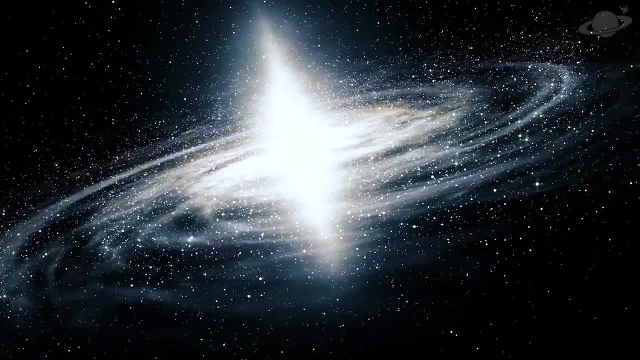 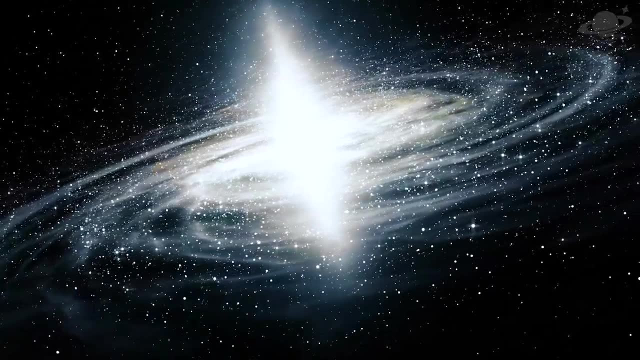 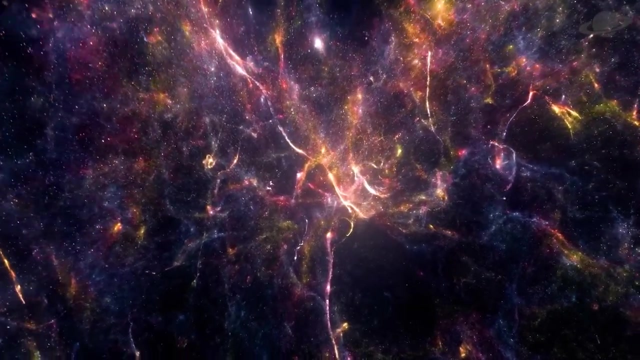 would be followed by another big bang, and the cycle would repeat. However, in the late 1990s, observations of type Ia- supernovae, extremely bright and distant stellar explosions- brought surprising new evidence. These observations not only confirmed that the universe is expanding, 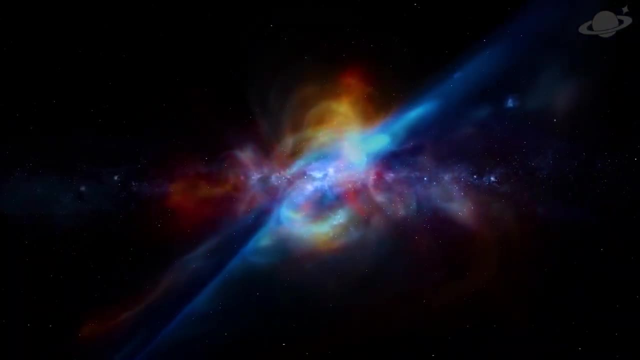 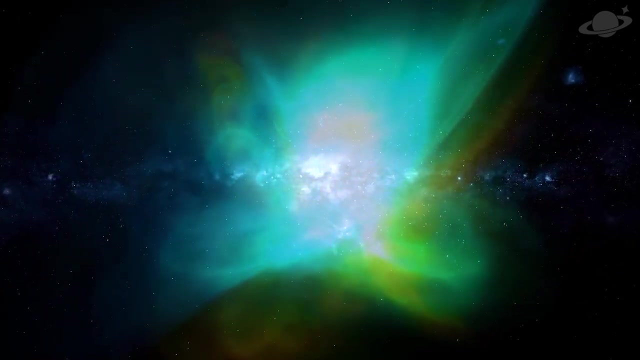 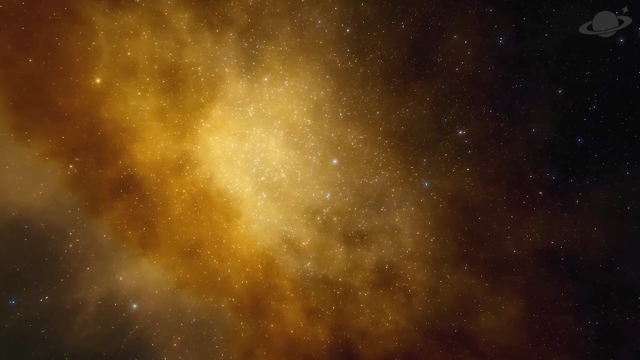 but also revealed that this expansion is speeding up. This acceleration hinted at the presence of a mysterious force called Dark Energy, which seems to oppose gravity, causing the universe to expand faster and faster. The discovery of Dark Energy marked a significant shift, leading to the prevailing theory of the Big Freeze, or Heat Death, According to. 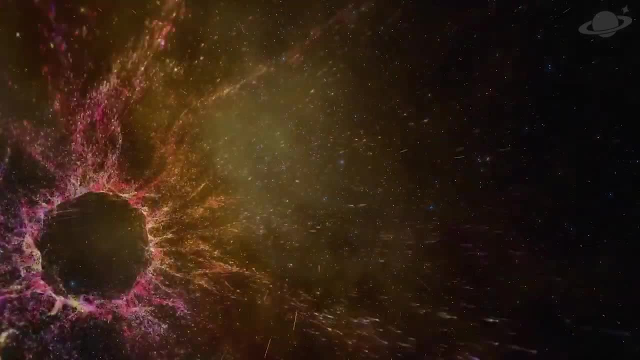 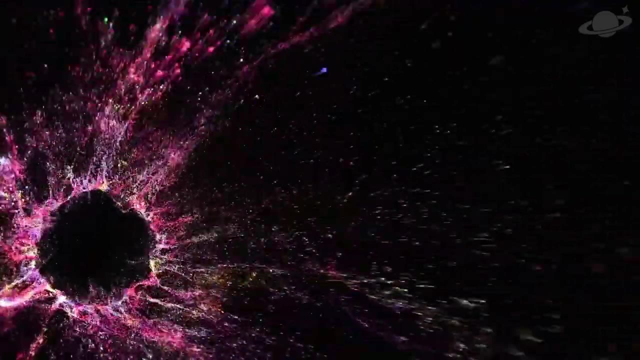 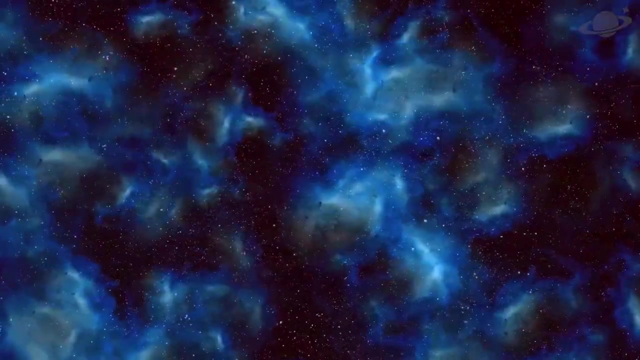 this theory, the universe will keep expanding endlessly Over trillions of years. energy will spread out more and more, causing the universe to gradually cool and dim. Additionally, modern cosmology has been transformed by detailed mapping of the cosmic microwave background radiation. This leftover radiation from the Big Bang offers crucial insights into the 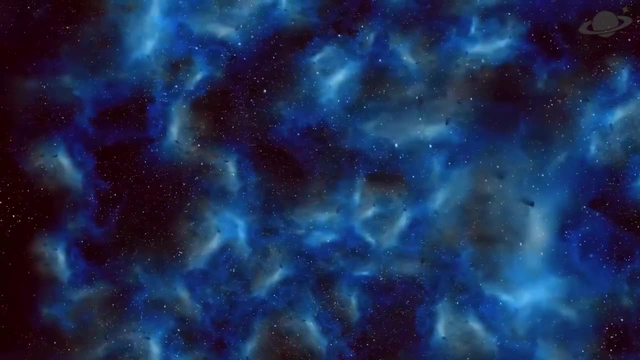 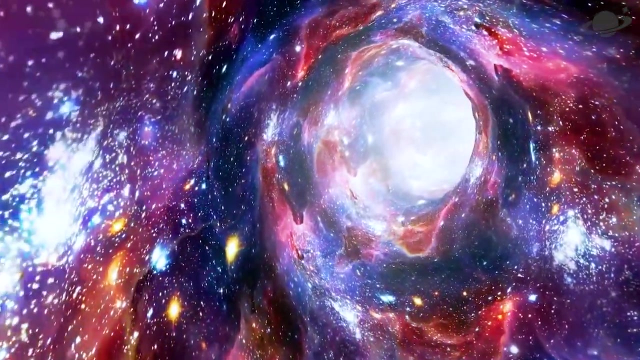 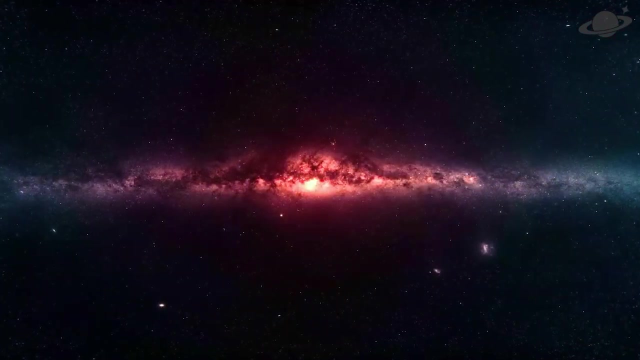 universe's early conditions and its subsequent evolution. Studies of the CMB support the notion of a flat and accelerating universe, supporting the Big Freeze idea. On the other hand, the Big Crunch theory offers a captivating and dramatic scenario for the universe's ultimate fate. 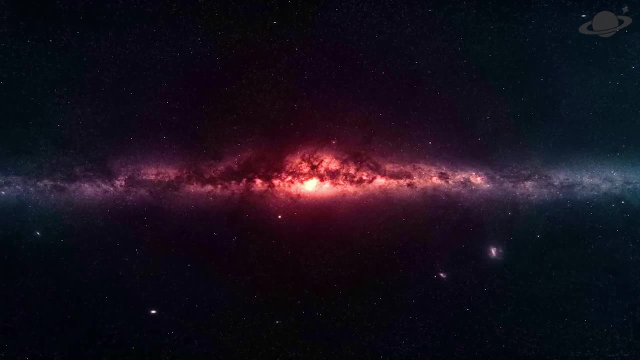 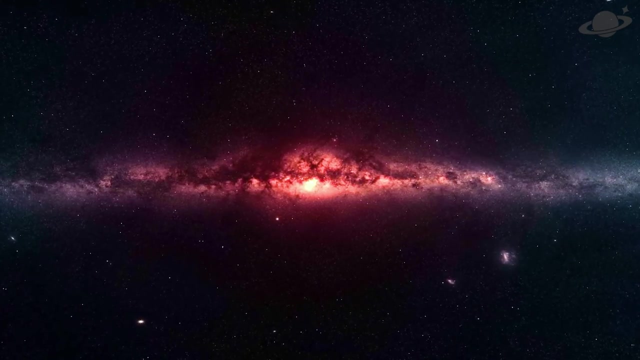 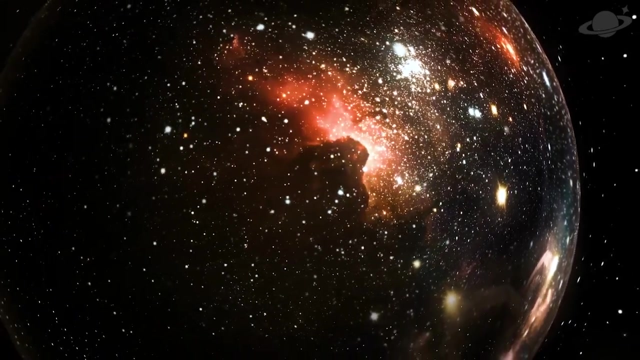 It presents a counterpoint to perpetual expansion rooted in the principles of gravity. According to the Big Crunch theory, the universe's expansion initiated by the Big Bang will eventually slow and reverse due to the gravitational attraction of all matter and energy. This 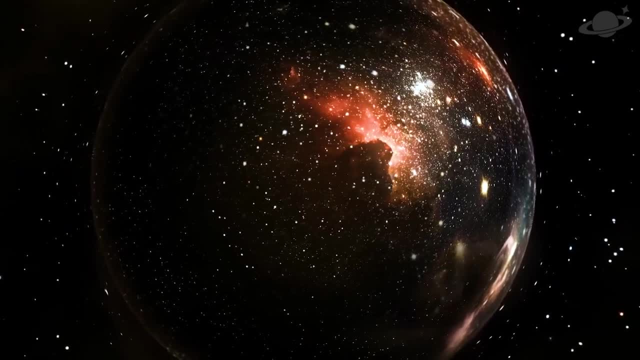 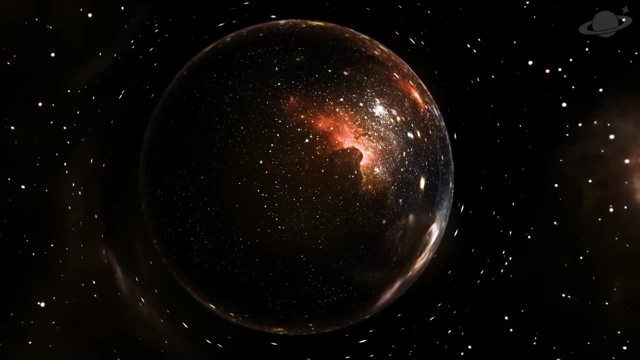 would result in a gradual collapse of the universe, pulling galaxies, stars and eventually all matter back toward a singular point. This theory draws upon principles from general relativity and the theory of gravity. This theory allows us to understand the universe's and posits that the universe's destiny is closely linked to its density. 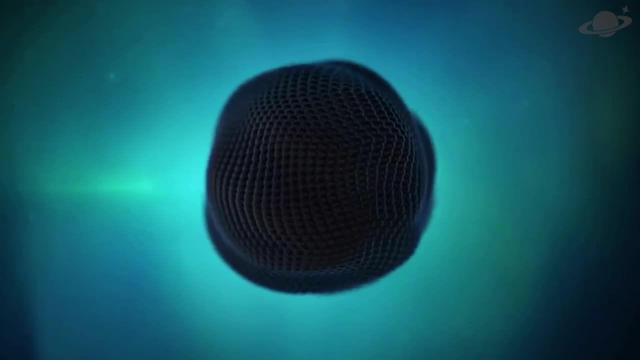 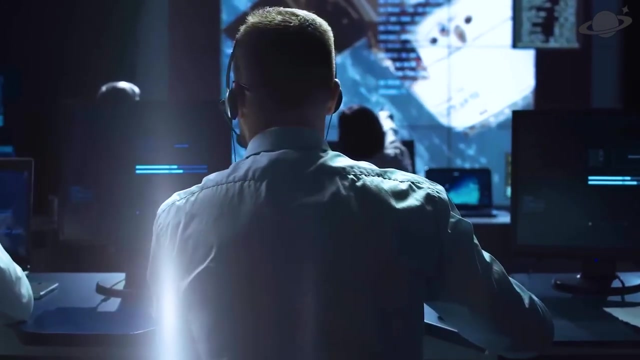 If the universe's density is high enough, all the gravity from stars, galaxies and other cosmic objects could eventually outweigh the force pushing them apart. This would cause the universe to stop expanding and start collapsing back in on itself As it contracts. temperatures would skyrocket. 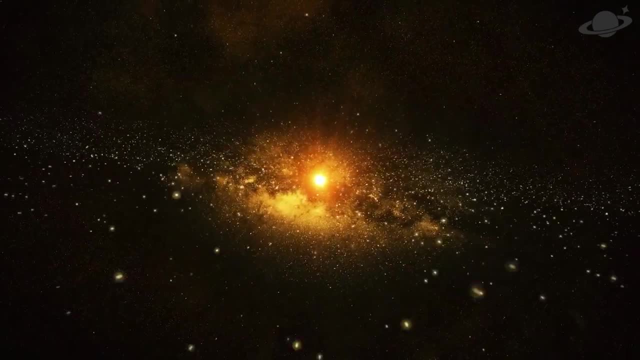 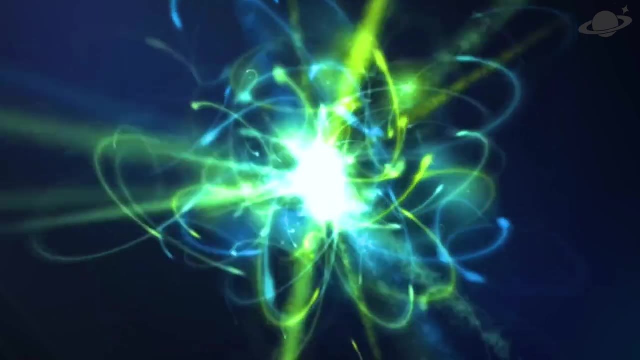 potentially undoing the effects of the Big Bang in a kind of cosmic rewind. The collapse known as the Big Crunch would end in a state of extreme density and heat, similar to the universe's early moments after the Big Bang. Some theories even suggest that this collapse could trigger another Big Bang. proposing a cycle where each collapse is followed by a new expansion phase. However, recent astronomical observations have cast doubt on the Big Crunch theory. The discovery of the universe's accelerating expansion implies that the influence of dark energy outweighs the gravitational pull of all matter. 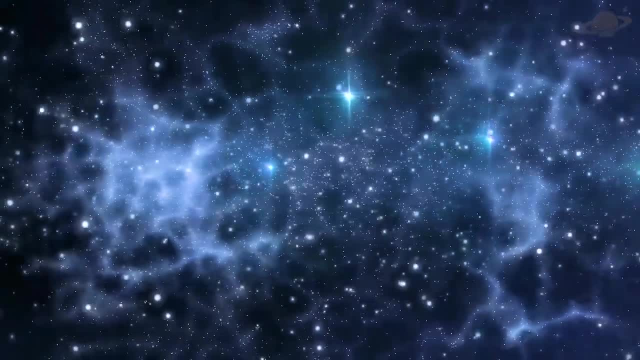 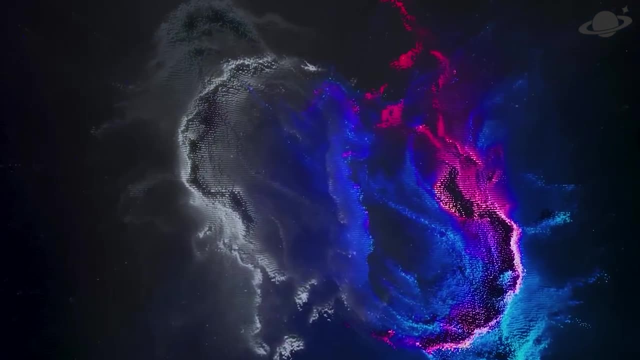 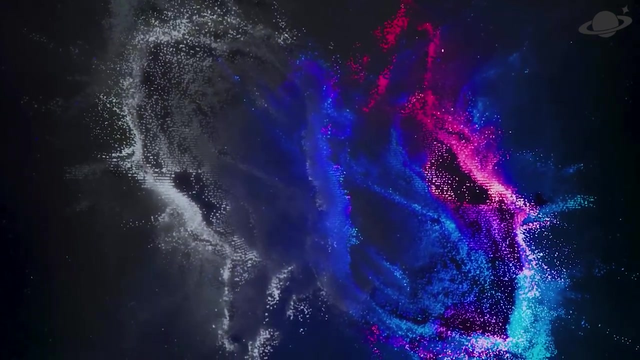 This suggests that the universe might keep expanding forever, making the Big Crunch scenario less likely according to current cosmological models. The Big Rip and the Big Crunch are two different theoretical scenarios for the universe's end, each with vastly different processes and outcomes. The Big Crunch involves the universe's gradual collapse. 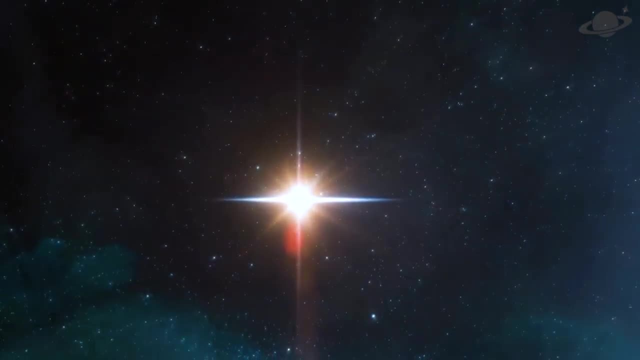 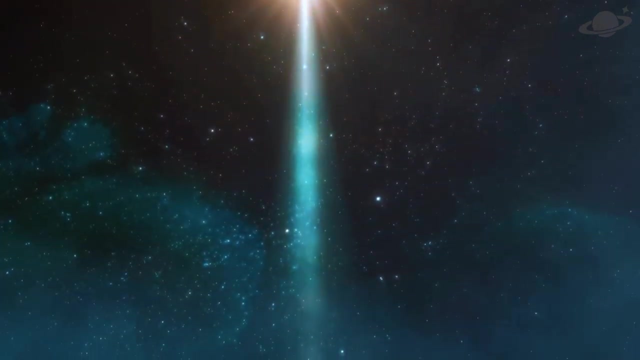 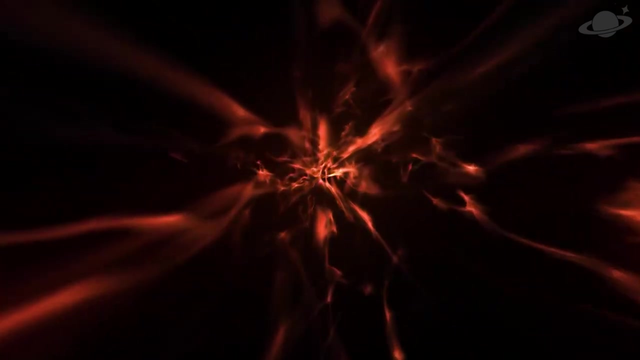 driven by the gravitational pull of matter and energy. If you're still watching, please like the video and turn on notifications for the channel so you don't miss our weekly documentaries. Moving on As the collapse progresses, everything in the universe gets compressed into a single incredibly dense point. This theory relies on the idea that the universe's density is high enough to counteract its expansion, aligning with principles from general relativity. However, it has become less favored due to observations indicating the universe's accelerating expansion. On the opposite end of the spectrum, we have the Big Rip theory. 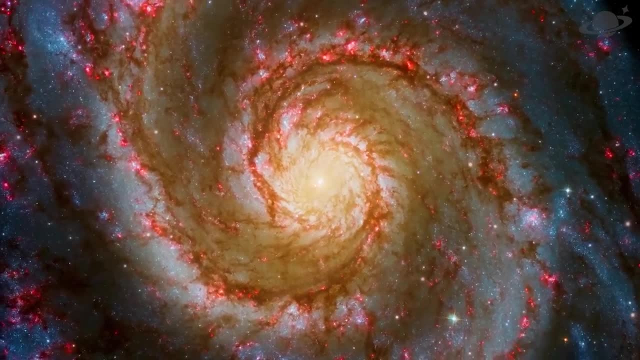 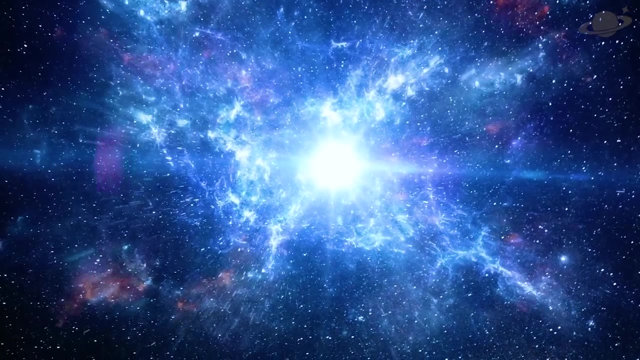 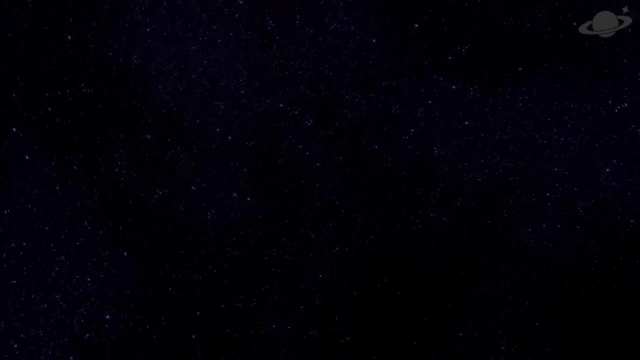 which suggests that the universe's expansion not only persists but speeds up indefinitely due to dark energy. Here, dark energy eventually becomes so dominant that it overwhelms all other forces, including gravity and electromagnetic forces that hold everything together, from galaxies down to atoms. 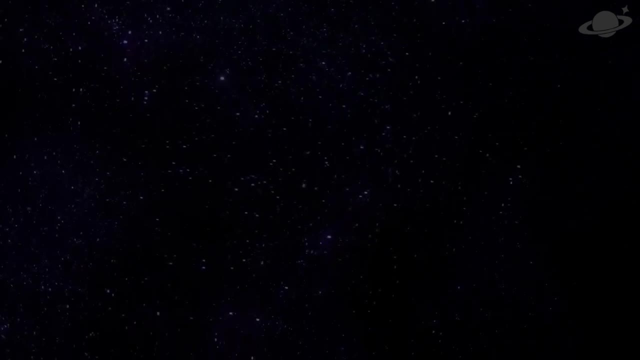 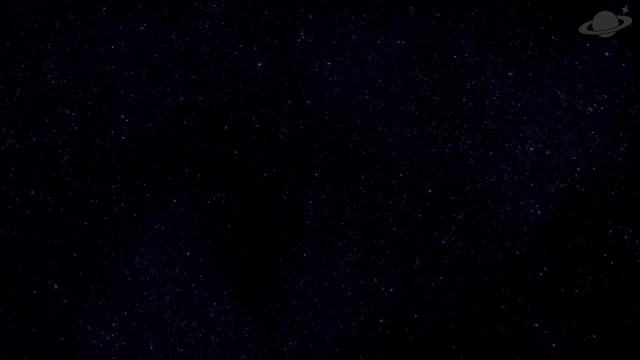 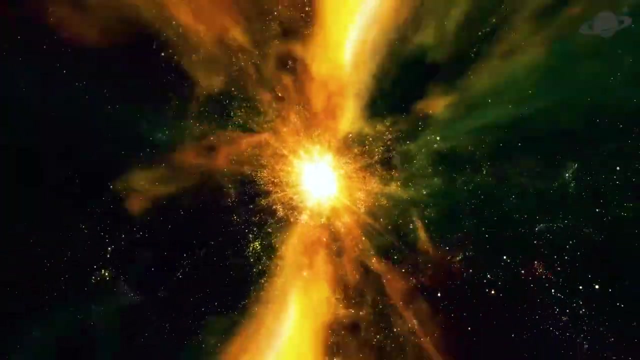 As the universe rapidly expands, it reaches a point where these fundamental forces can't keep structures intact anymore. Galaxies would tear apart, followed by the breakup of individual star systems, planets and, eventually, the very essence of matter itself. The Big Rip ends with the universe torn apart at its most basic level. 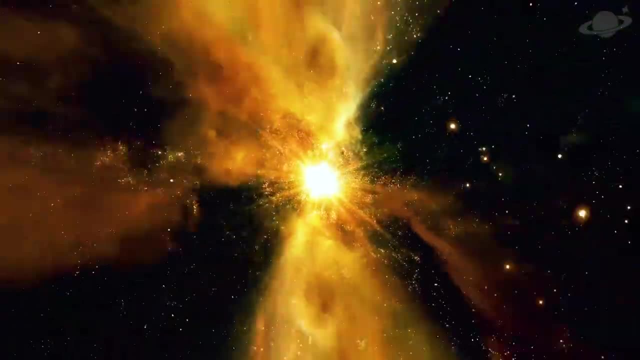 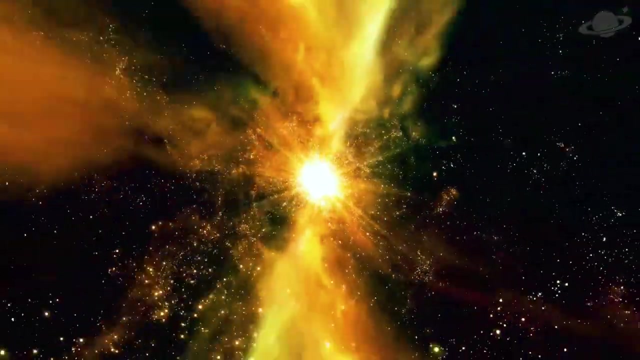 resulting in a sparse, cold and dark state with particles scattered far apart. The main contrast between the two theories lies in their driving forces. The Big Crunch is pushed by gravity, leading to a collapse, while the Big Rip is propelled by a relentless acceleration. 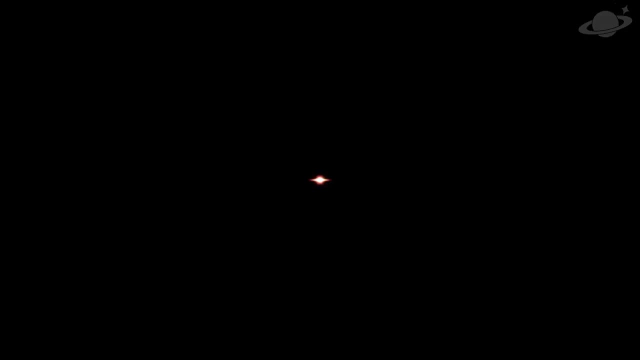 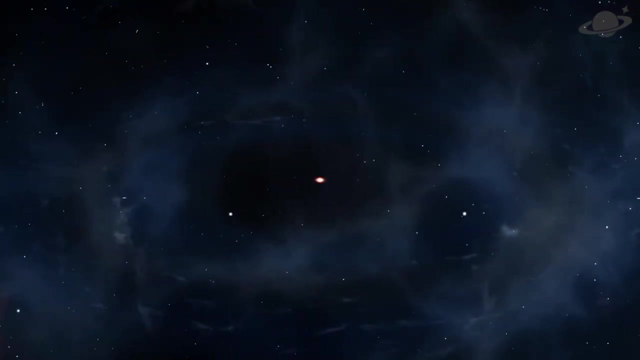 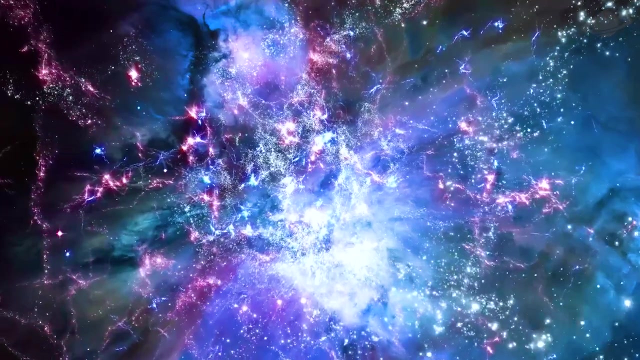 of the universe's expansion due to dark energy. Furthermore, the timelines for these events differ greatly. The Big Rip would happen relatively quickly once it gains momentum, unlike the Big Crunch, which would unfold over a longer period. Both theories showcase the intricate and ever-changing nature of the universe. 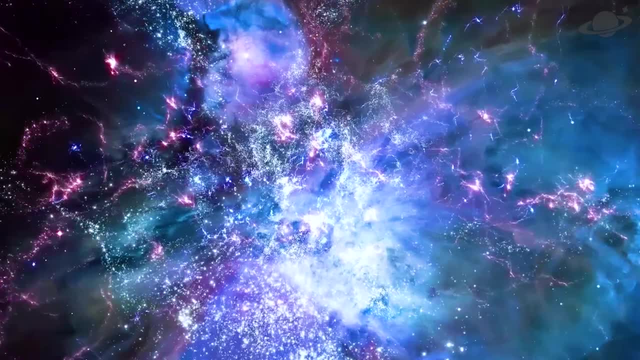 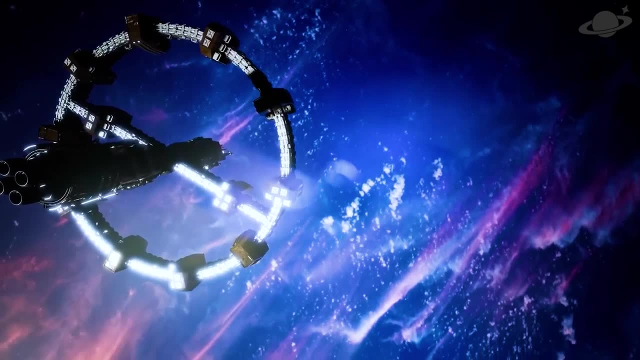 offering different viewpoints on how its story might conclude. While current observations hint that a Big Rip might be more plausible than a Big Crunch, these are still speculative ideas in cosmology. Now let's talk about the concept of heat death, also known as the Big Freeze. 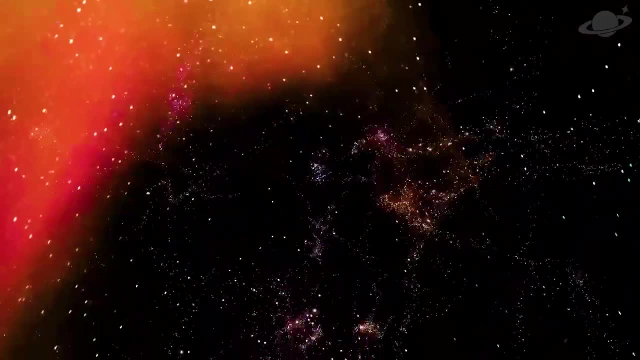 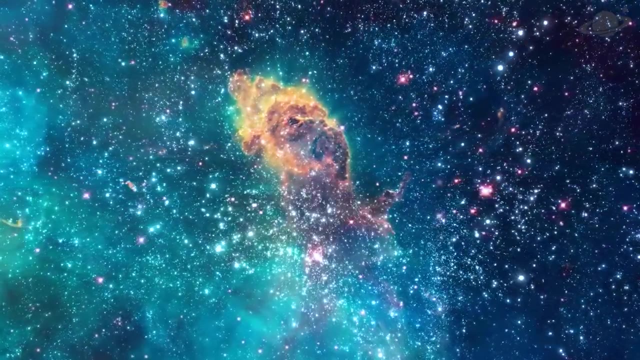 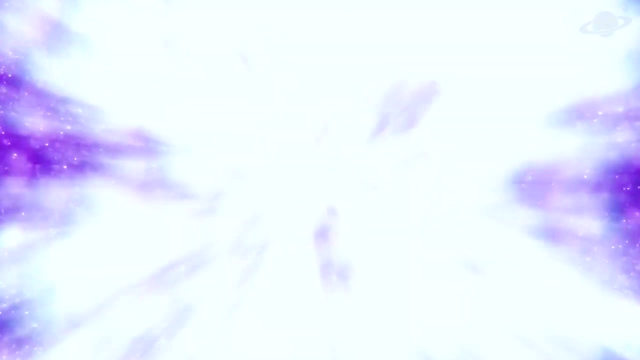 This idea is rooted in thermodynamics, specifically the second law, which says that the total disorder or entropy of a closed system can't decrease over time. In the universe's context, this means that entropy keeps rising until it reaches a peak. The heat death scenario envisions a future where the universe expands so much. 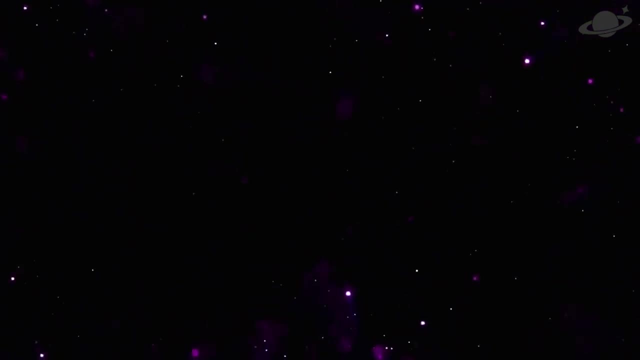 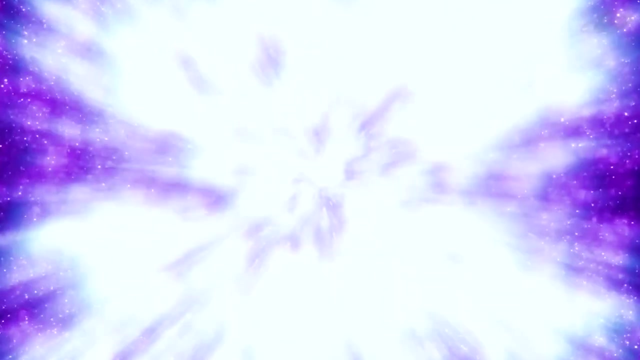 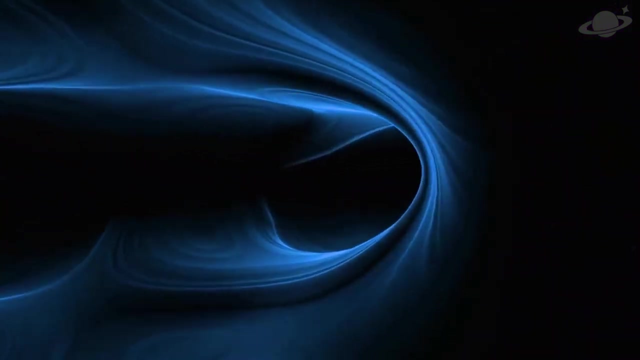 that all energy is evenly spread out. This uniform energy distribution results in no thermodynamic free energy, meaning no more useful work can be extracted from the system. In simpler terms, it's like a battery fully drained of power and unable to recharge. In this scenario, stars will run out of fuel and stop shining. 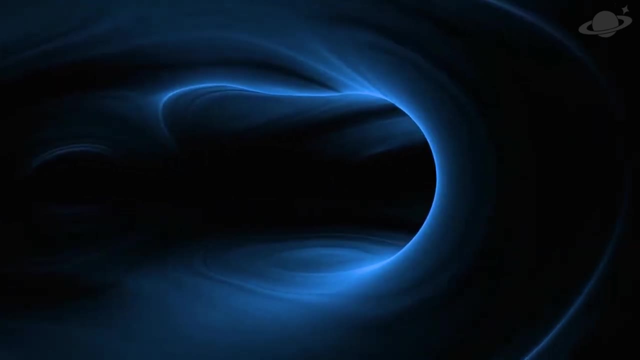 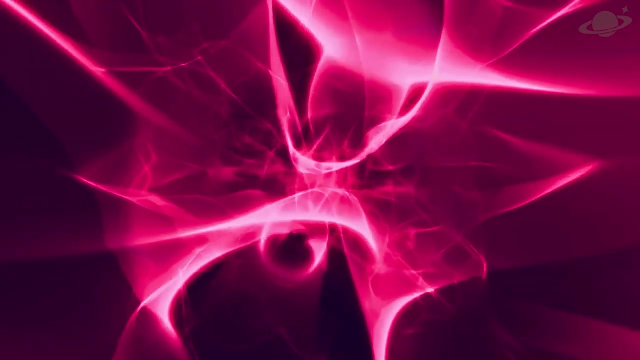 leaving behind remnants like white dwarfs, neutron stars and black holes. Eventually, even these remnants will fade away, with black holes evaporating due to Hawking radiation, Galaxies will drift apart and the universe will become vast, cold and dark. 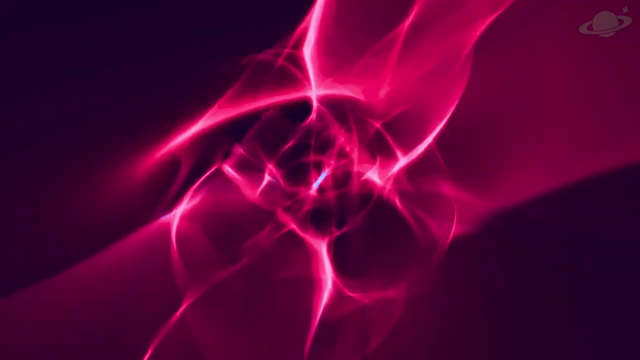 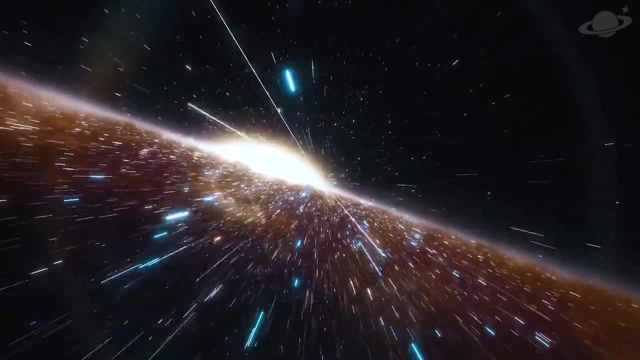 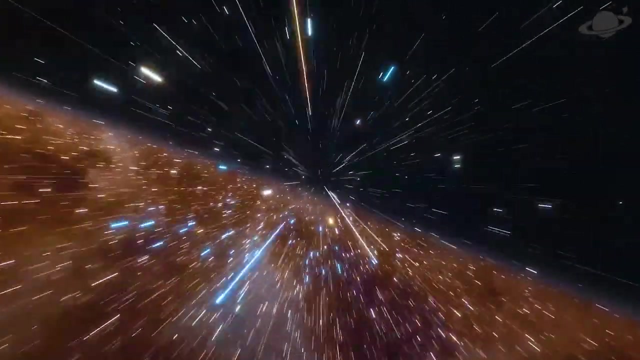 Temperature differences, which drive energetic processes, will disappear. Without these variations, no energy transfer can happen, leading the universe to a state of maximum disorder and equilibrium. At this point, all known physical processes would stop. The heat death scenario is seen as the most probable outcome based on current cosmological models. 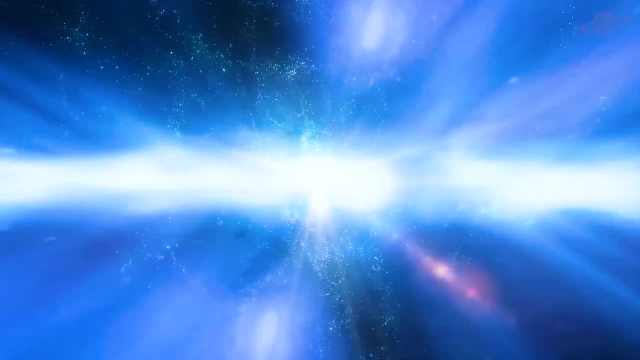 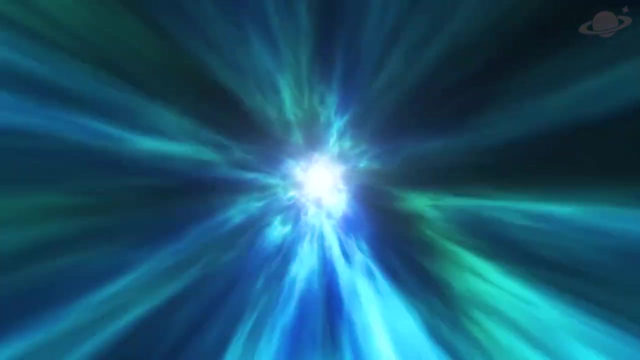 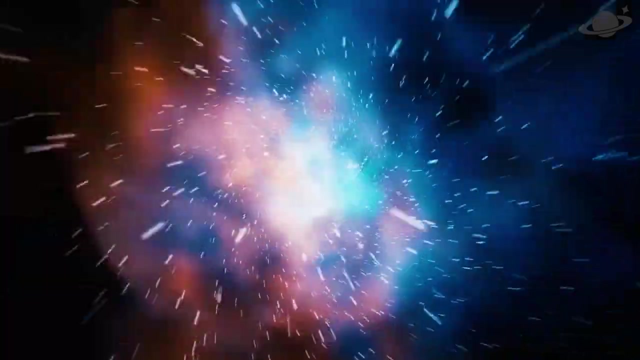 which consider the universe's observed accelerated expansion. This expansion, fueled by dark energy, suggests that the universe will keep growing, eventually dispersing all matter and energy. Black holes, mysterious and powerful cosmic entities, are key players in theories about the universe's end. 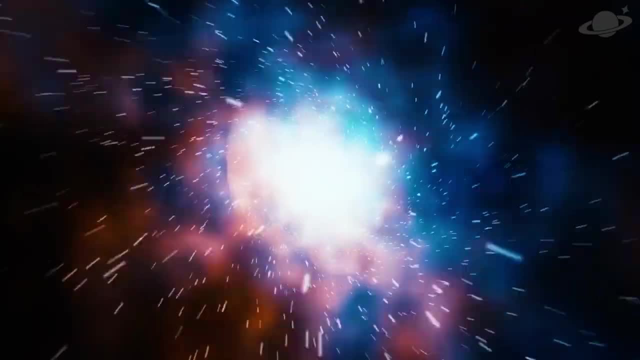 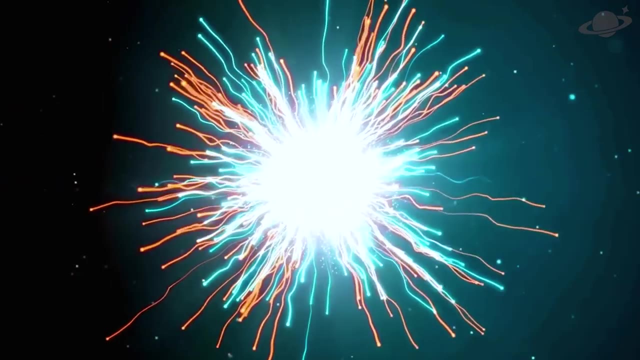 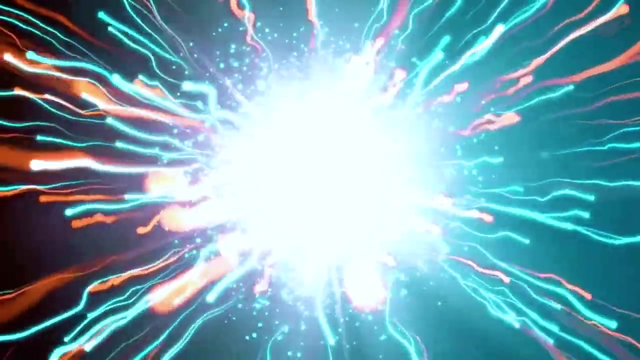 Their unique characteristics offer insights into the universe's long-term fate. In the Big Crunch theory, black holes could hasten the universe's collapse. by exerting significant gravitational pull, They might merge and grow larger, accelerating the universe's contraction towards a denser state. 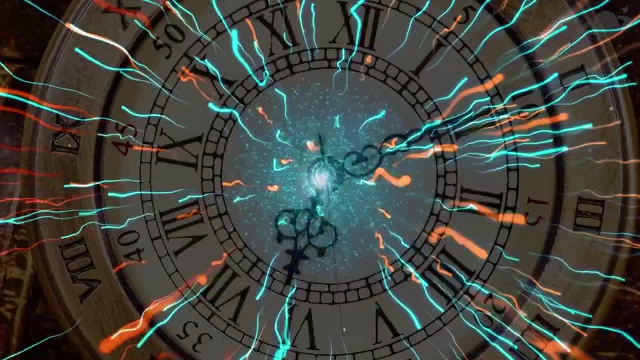 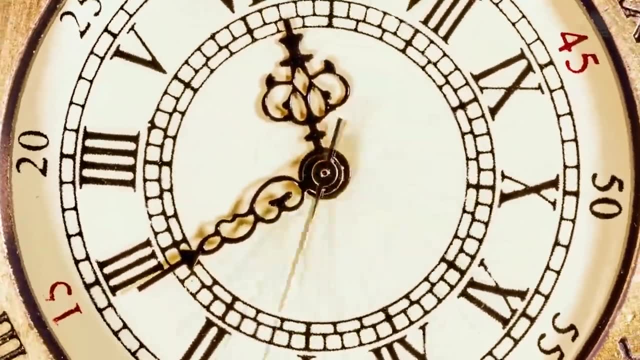 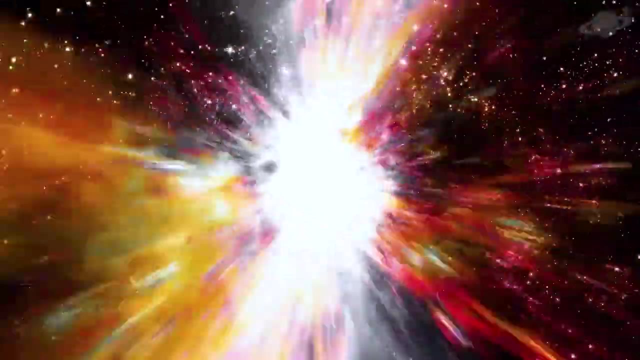 However, in the heat death scenario, black holes mark one of the universe's final stages. After stars die out and galaxies disperse, black holes remain Over vast time spans. even black holes evaporate, emitting Hawking radiation. This process is slow but inevitable, contributing to the eventual dispersal. 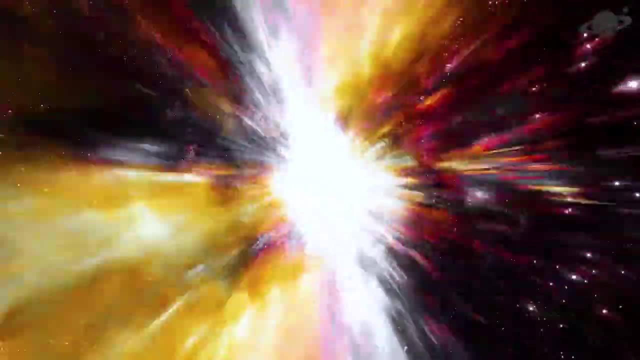 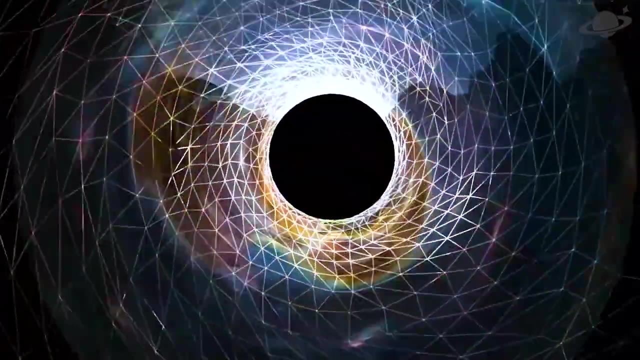 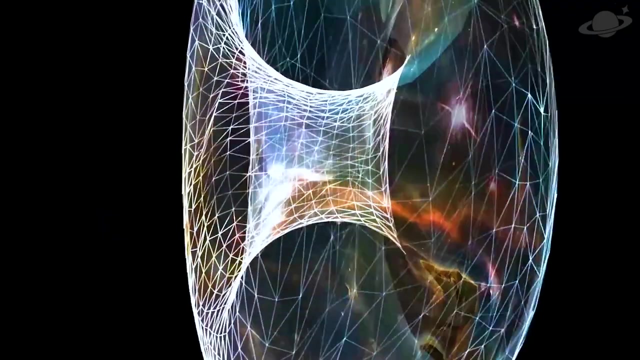 of all matter and energy. As black holes evaporate, they gradually lose mass until they disappear entirely. This slow evaporation could be one of the last events in the heat death scenario for the universe. As black holes emit Hawking radiation, they contribute to the universe's increasing disorder. 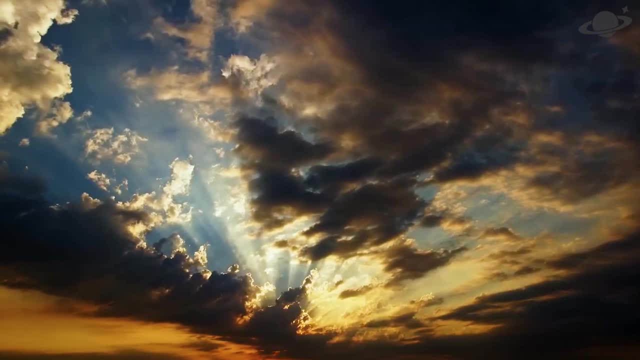 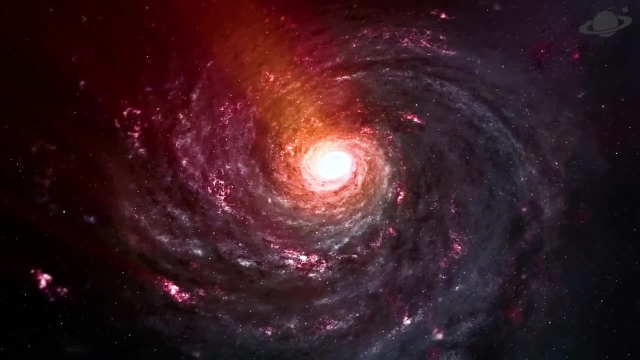 When the last black hole vanishes, the universe would be left extremely cold, with almost no energy and lacking any significant structure, a stark contrast to its fiery and diurnal state. This is a dynamic beginning, Studying black holes and their characteristics, like event horizons and singularities. 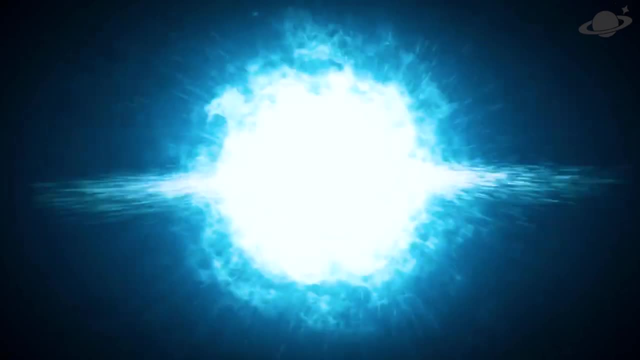 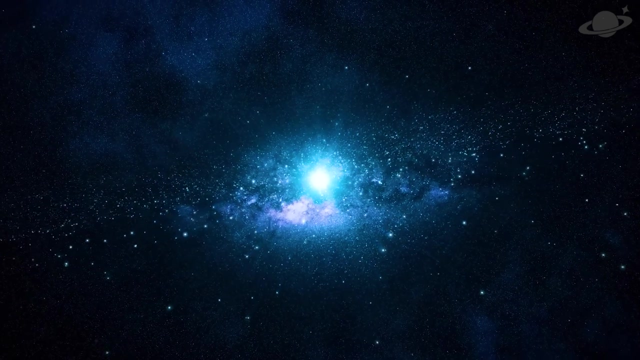 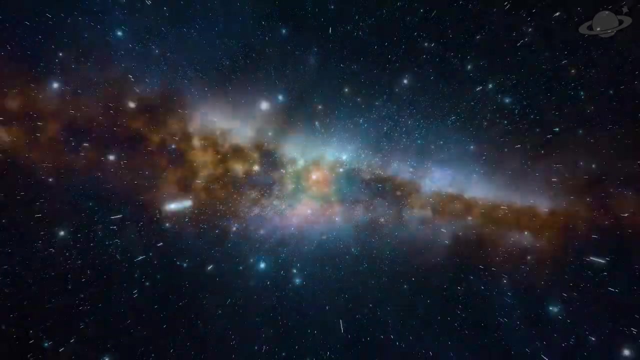 helps us understand the fundamental nature of space-time and quantum mechanics. These understandings are crucial for developing a more complete theory of the universe's fate, especially in bridging the gap between general relativity and quantum physics. Dark energy: a mysterious force captivating scientists and the public alike. 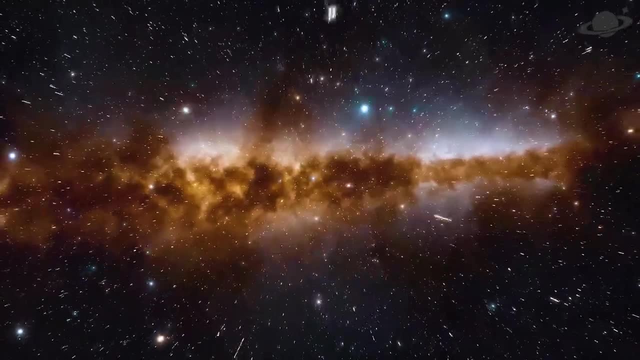 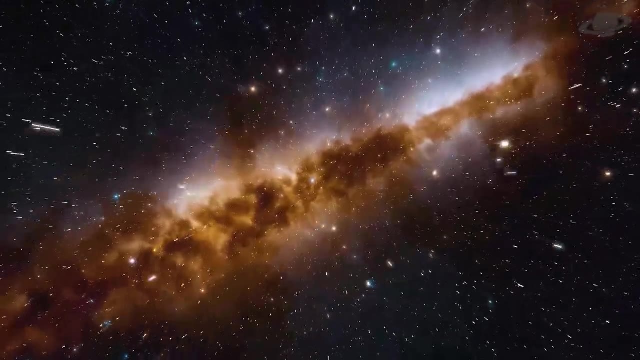 plays a vital role in determining the universe's future. It's a type of energy present throughout space that speeds up the universe's expansion. Scientists first inferred its existence from observations of distant type Ia supernovae in the late 1990s. 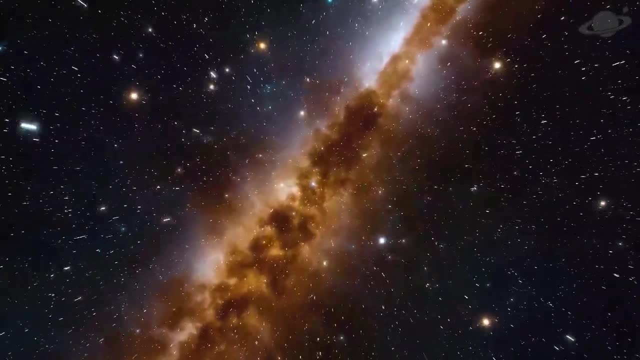 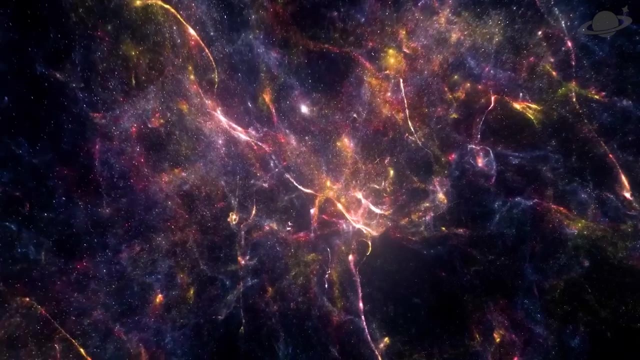 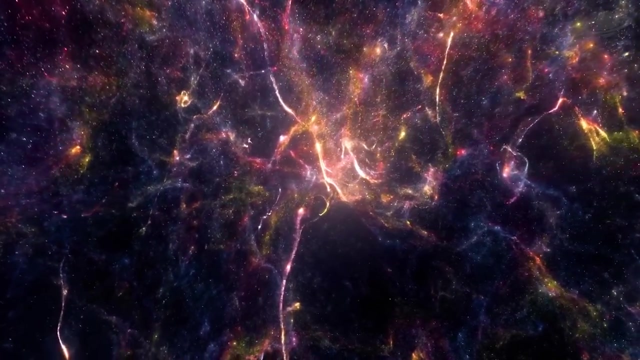 These observations showed that the universe's expansion rate is actually increasing over time. contrary to previous beliefs, Known forces of gravity acting on visible matter alone couldn't explain this acceleration, leading to the hypothesis of dark energy as an unknown repulsive force. Dark energy is one of the biggest mysteries in modern cosmology. 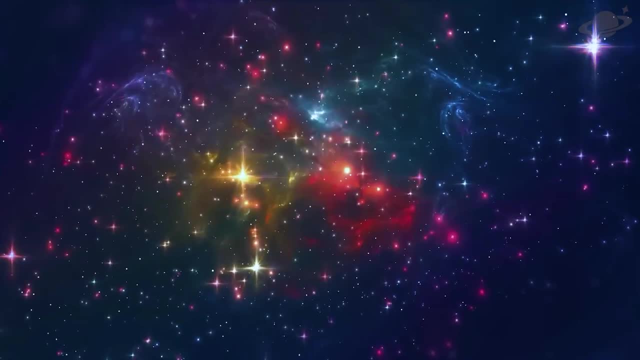 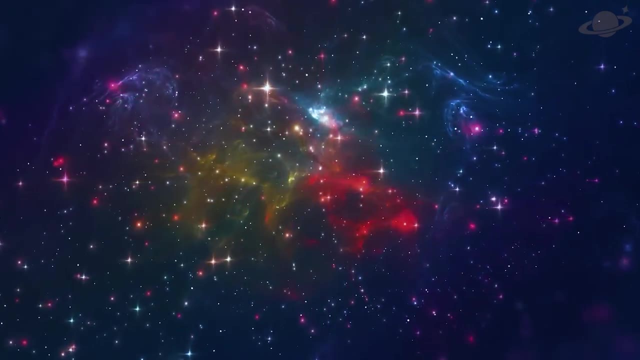 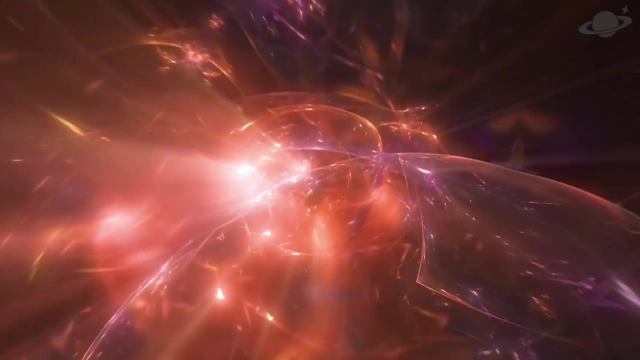 It's invisible and doesn't interact with light, making it super tricky to spot directly. Scientists have come up with different theories to explain it, from ideas like Albert Einstein's cosmological constant to more complex concepts involving new fields and particles. Dark energy is super important for the future of the universe. 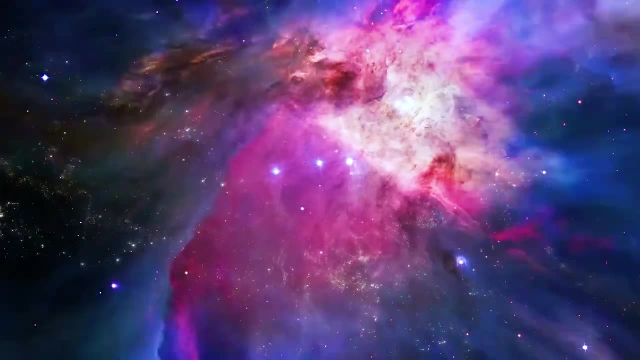 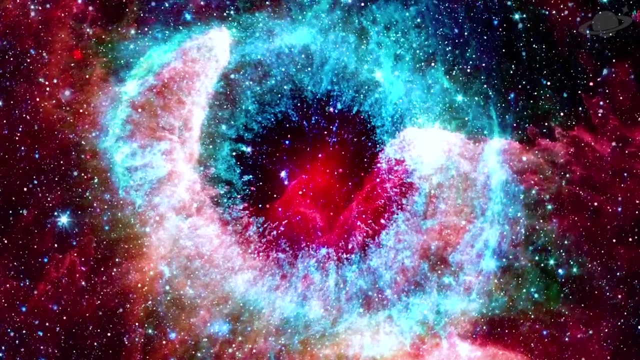 If it keeps on being the main source of energy, like current observations suggest, it's going to have a huge impact on what happens next. Dark energy's push is making the universe expand faster and faster, leading to possibilities like the Big Rip or the Heat Death. 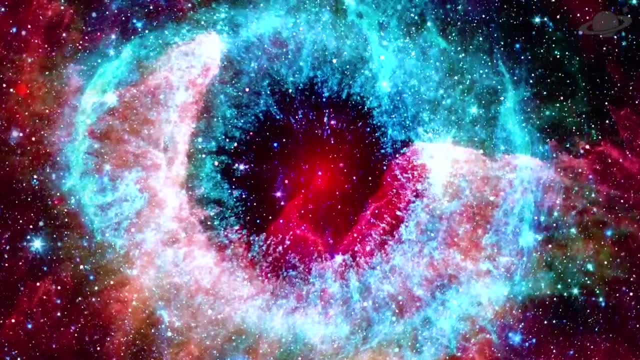 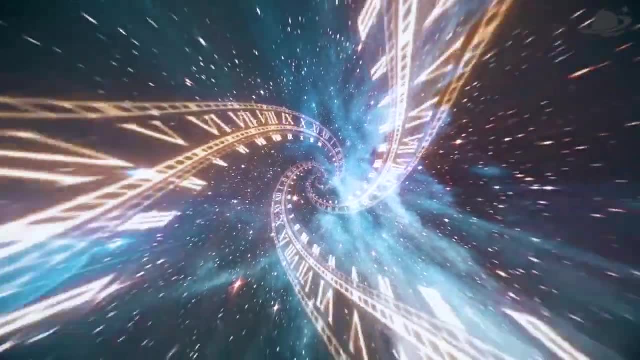 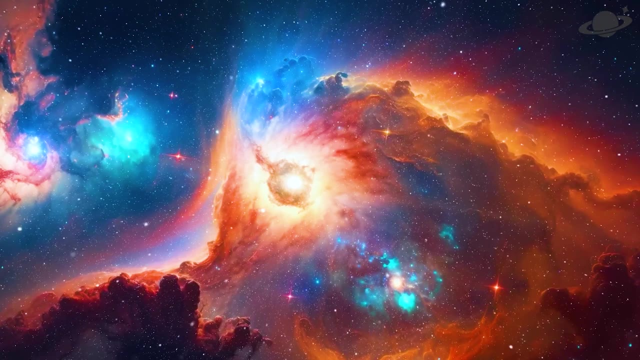 In the Big Rip scenario, this push gets so strong that it tears everything apart: galaxies, stars, planets, even atoms. In the Heat Death scenario, the ongoing expansion makes the universe colder and emptier as stars and galaxies move farther away and lose their energy. 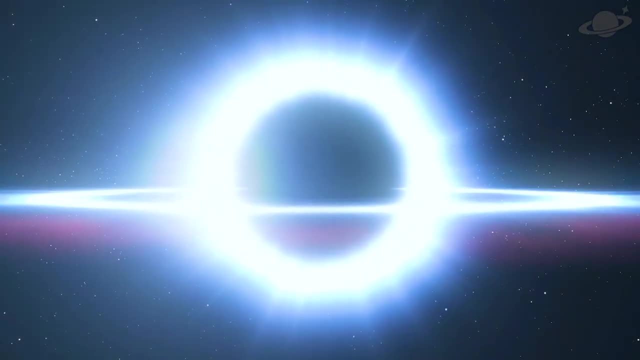 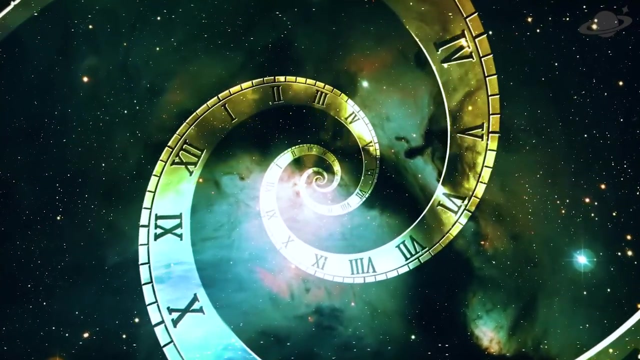 With dark energy calling the shots, the universe might just keep on expanding forever, getting bigger, colder and lonelier as time goes on. This marks a shift from earlier ideas like the Big Crunch, where the universe's expansion would eventually halt and reverse. 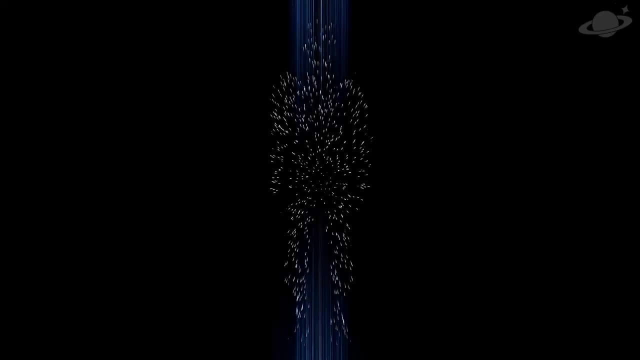 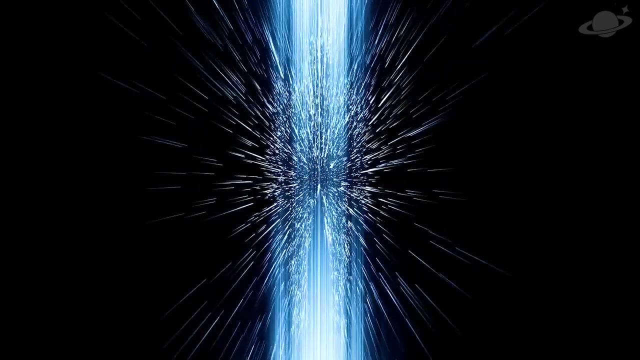 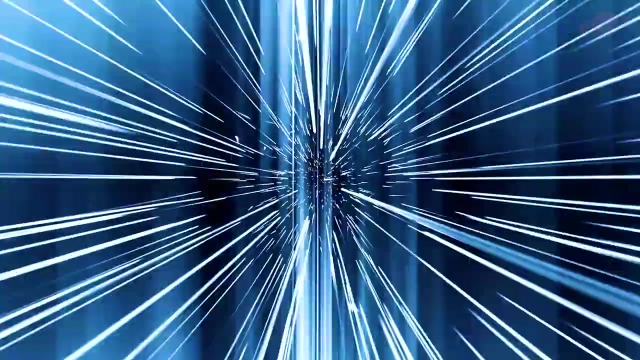 But how do we measure the universe's expansion rate? Measuring this rate, known as the Hubble constant, is a fascinating process that involves advanced technology and keen astronomical observations. One primary method involves looking at the redshift of distant galaxies, As galaxies move away from us due to the universe's expansion. 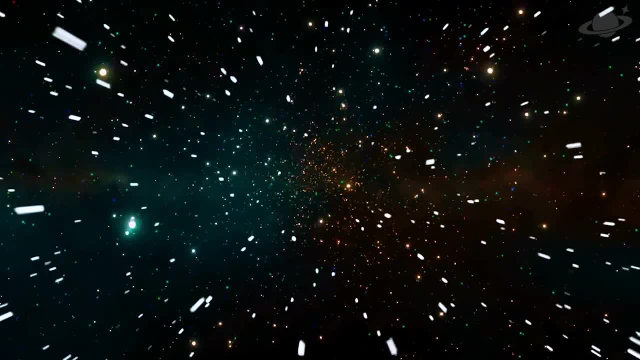 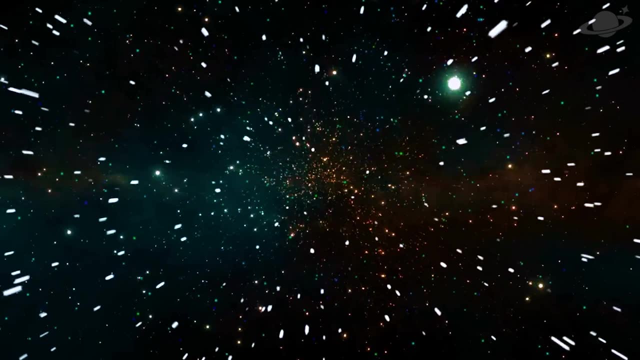 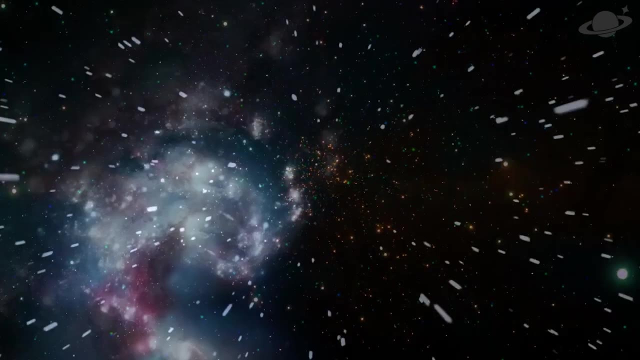 the light they emit shifts towards the red end of the spectrum. By measuring this redshift, astronomers can figure out how fast these galaxies are moving away from us. To determine the universe's expansion rate, astronomers use specific objects called standard candles. These are objects like Type Ia supernovae, which explode with a consistent brightness. 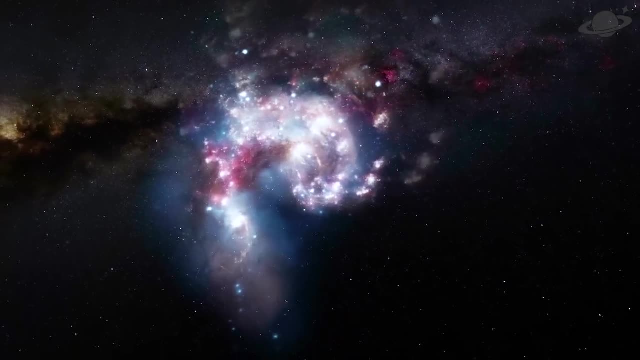 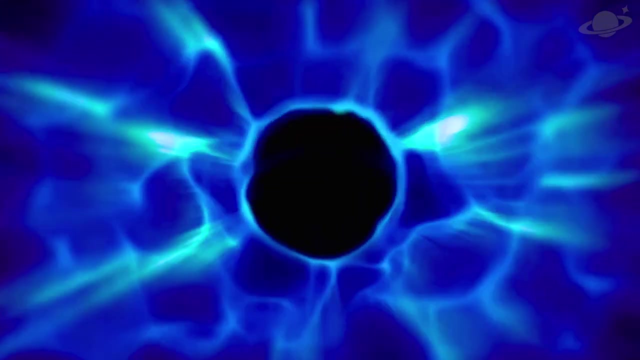 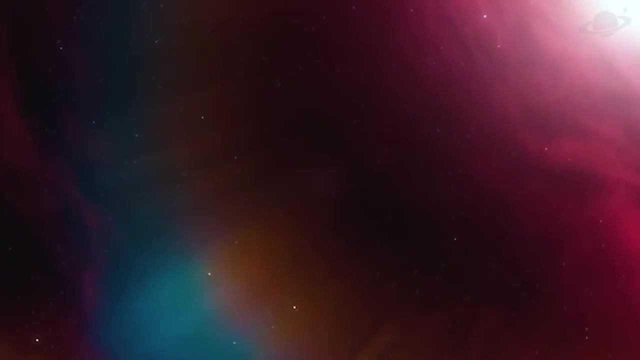 By observing how bright these supernovae appear from Earth, scientists can estimate their distance. The farther they are, the fainter they appear. Similarly, sea-feed variables, a type of star with a predictable brightness pattern, serve the same purpose By measuring these distances and matching them with the speed of galaxies' movement. 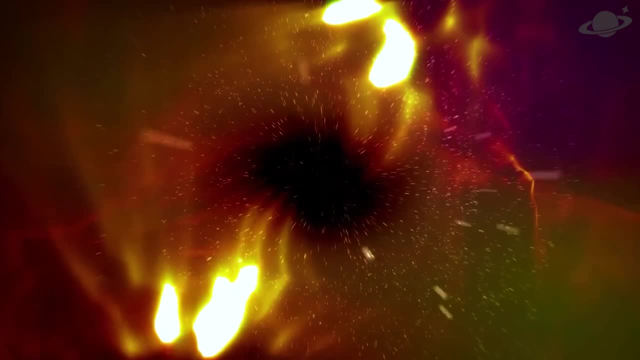 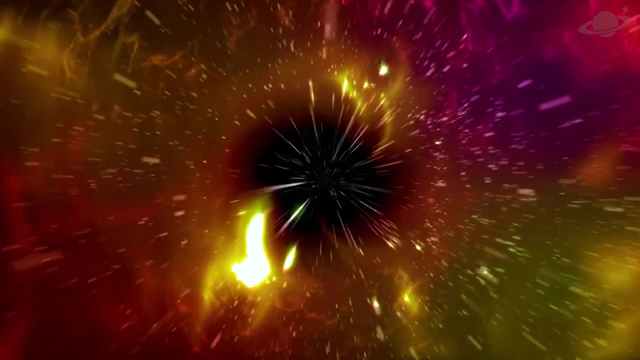 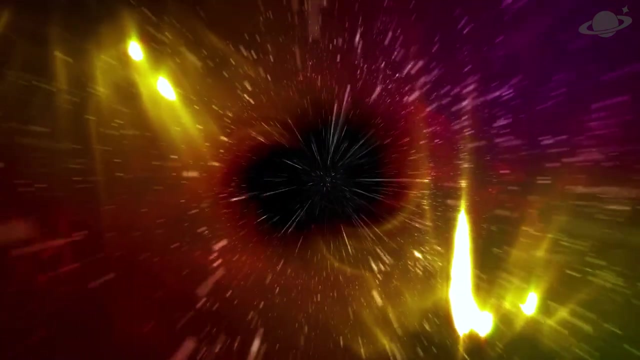 astronomers can work out the universe's expansion rate. Another method involves studying the cosmic microwave background – the leftover radiation from the Big Bang. By analyzing the CMB's small temperature changes, astronomers can figure out various aspects of the universe, including its expansion rate. 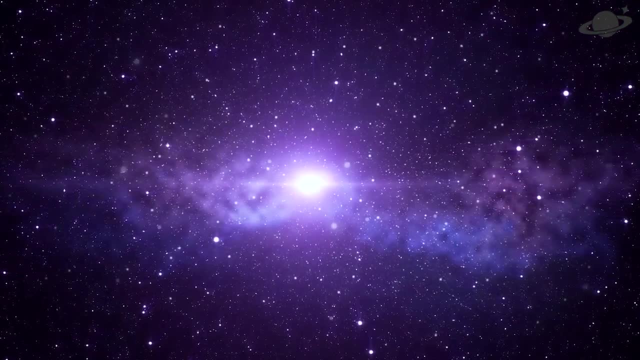 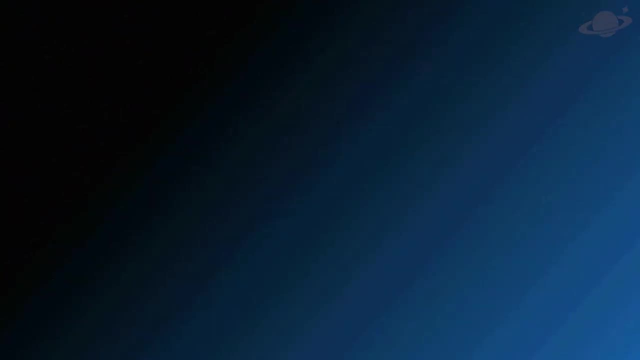 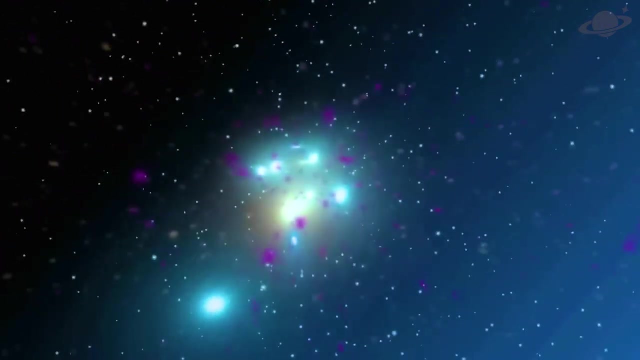 This approach gives us a peek into the universe's early days, which offers a different angle from studying far-off galaxies today. Also, baryon acoustic oscillations- regular periodic patterns in how visible matter is spread out- come into play. By examining these patterns and the universe's large-scale structure, 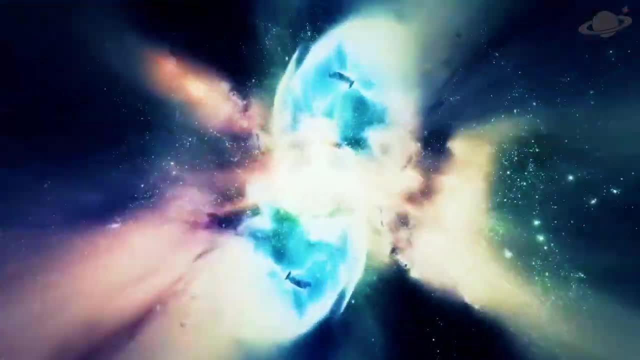 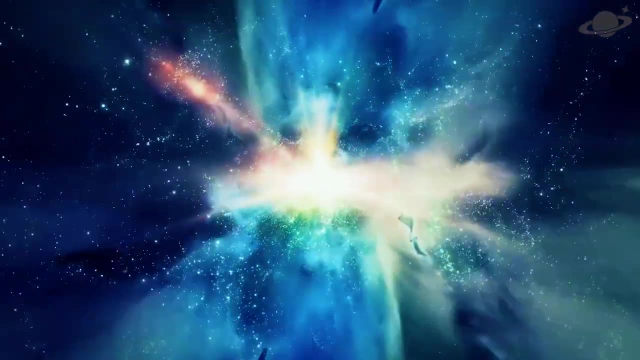 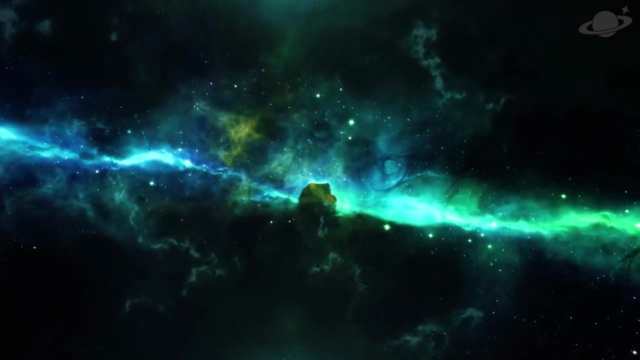 astronomers can figure out how quickly the universe was growing at different times in its history. There's also a newer method called gravitational lensing that helps with these measurements. This happens when a massive object, like a cluster of galaxies, bends the light from things behind it because of its gravity. 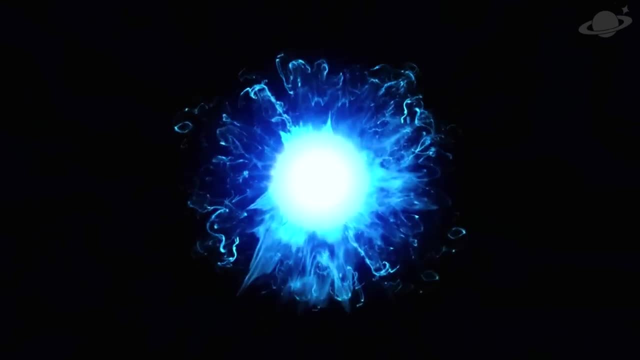 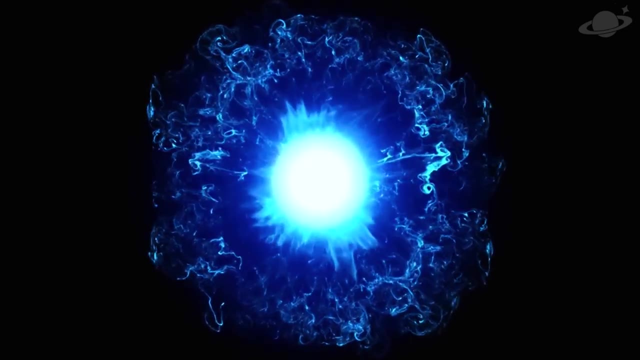 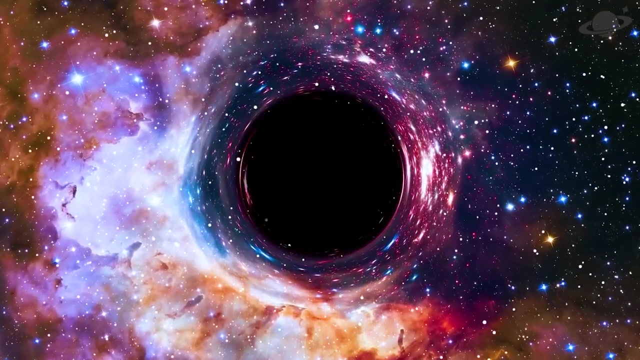 How much the light bends can tell us about how fast the universe is expanding, based on the universe's shape, which is influenced by its expansion rate. Each method has its own complexities and limits. Interestingly, they sometimes give slightly different answers for the Hubble constant. 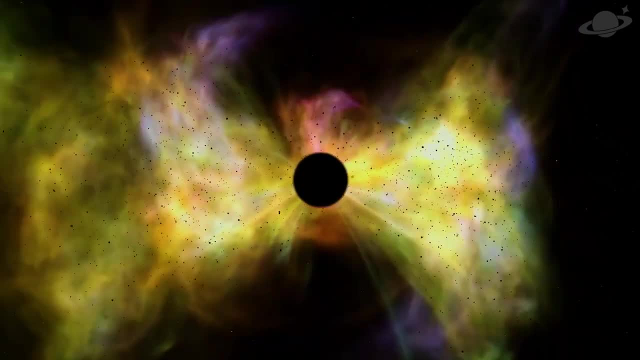 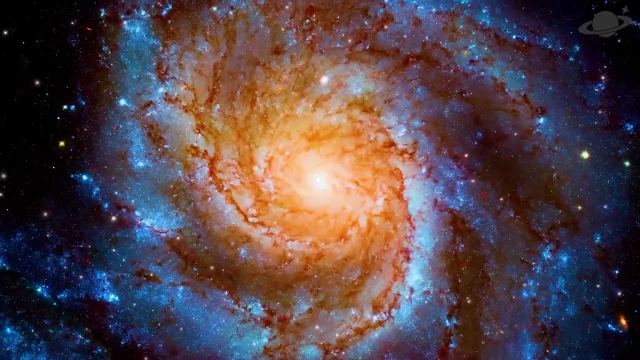 which has caused a bit of confusion in cosmology, called the Hubble tension. Quick reminder to subscribe, if you haven't already, so you can keep up with our future astronomy documentaries. Thank you so much. Now let's talk about dark matter's role in the universe's end. 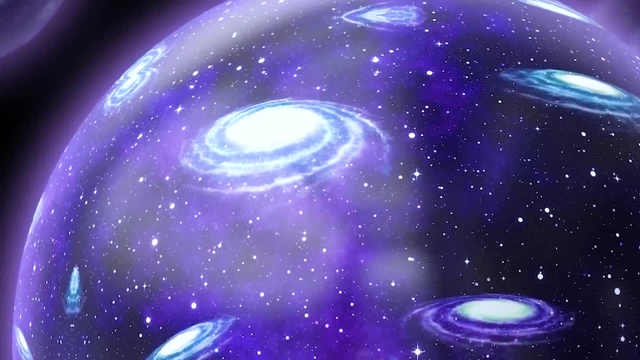 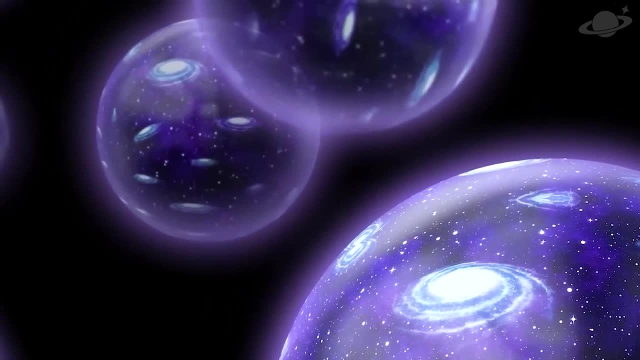 Dark matter, a mysterious but crucial part of the universe, is key in theories about how the universe will end. Even though we can't see dark matter and it doesn't give off or absorb light, we know it's there because of its gravity's effects on things we can see, like stars and galaxies. 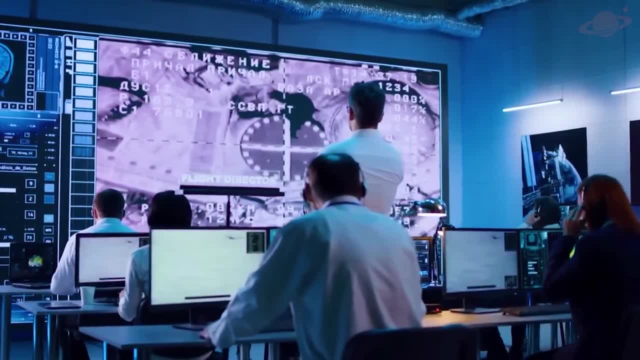 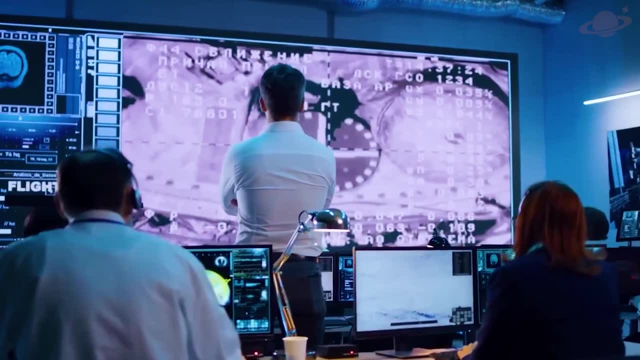 Understanding dark matter is vital for predicting what will happen in the end In the big picture of the universe's fate. dark matter's main influence comes from its gravity. This mysterious stuff makes up about 27% of the universe's total mass and energy. 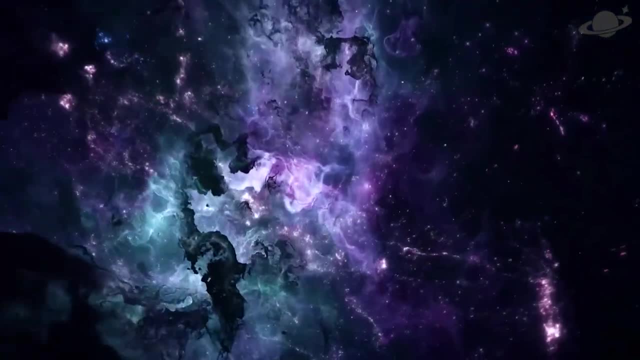 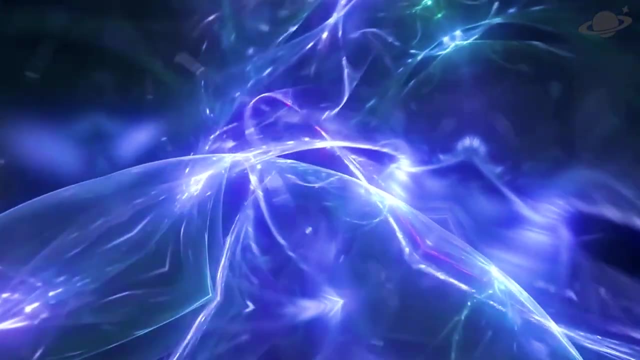 way more than the regular stuff we see, like stars and planets. Its gravity has been super important in shaping how the universe is structured, pulling stuff together to form galaxies and groups of galaxies. In scenarios like the Big Crunch, dark matter's gravity could be a big deal. 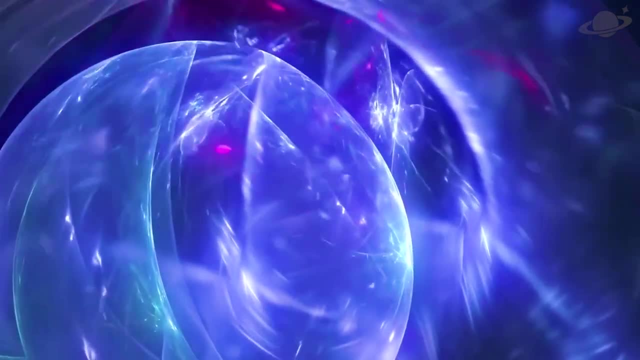 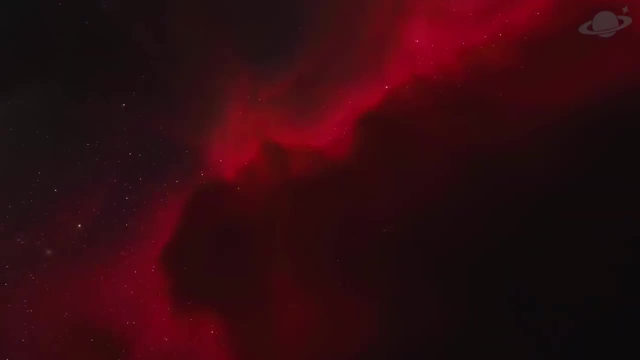 If dark matter's pull is strong enough to counteract the universe's expansion caused by dark energy, it could make the expansion stop and even reverse. In such a situation, the universe would stop getting bigger and start getting smaller, eventually squeezing all matter into one tiny, super-dense point. 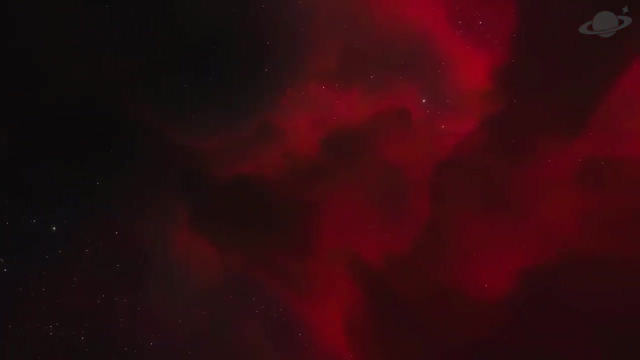 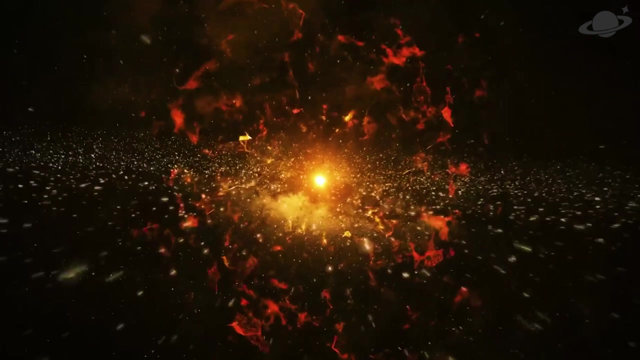 But recent observations, especially of how the universe's expansion is speeding up, suggest that dark energy's push is stronger than dark matter's pull. This makes the Big Crunch scenario less likely for now. In the heat death idea, dark matter still plays a role. 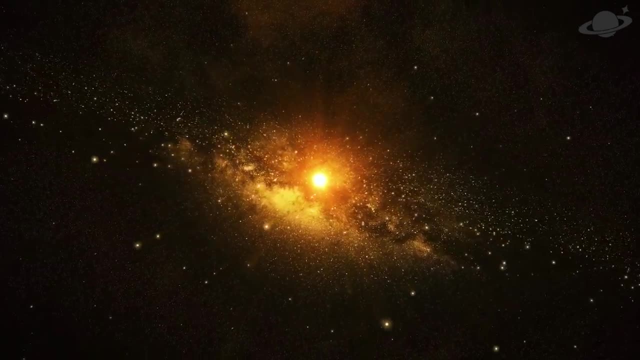 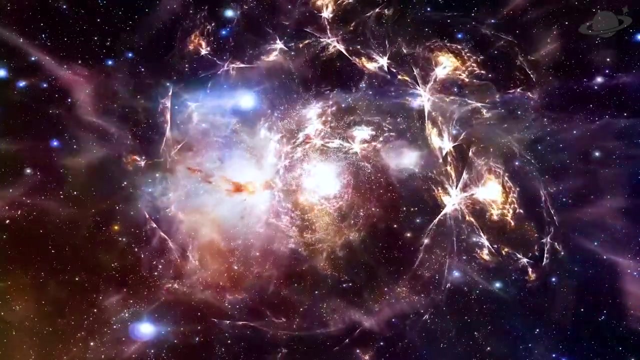 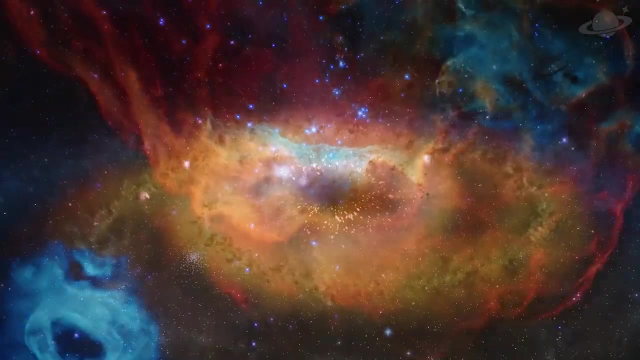 But it's not as active. As the universe stretches out and cools down, dark matter, just like regular stuff, spreads out more thinly. Its gravitational pull weakens as galaxies and groups of galaxies move farther apart. In a universe headed for heat death, dark matter sticks around. 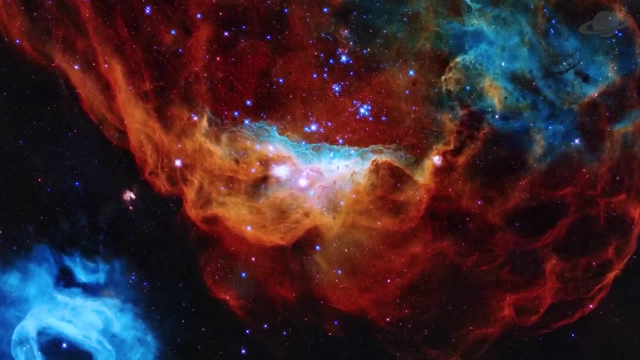 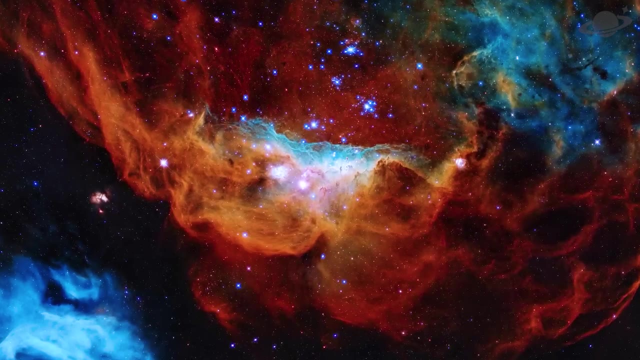 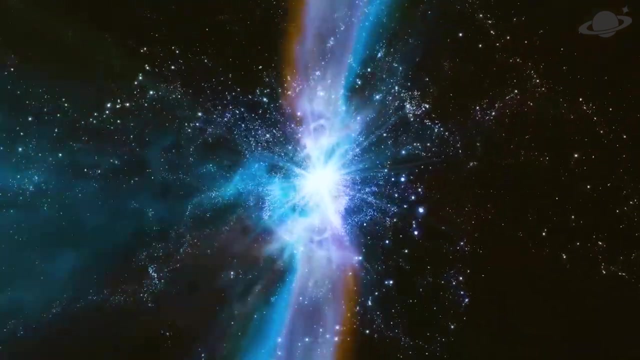 But its power to shape how the universe looks and works fades away over time. Understanding dark matter's part in the universe's end helps us grasp how the universe changes and grows over time. It's like a cosmic support structure shaping how galaxies and groups of galaxies form and move. 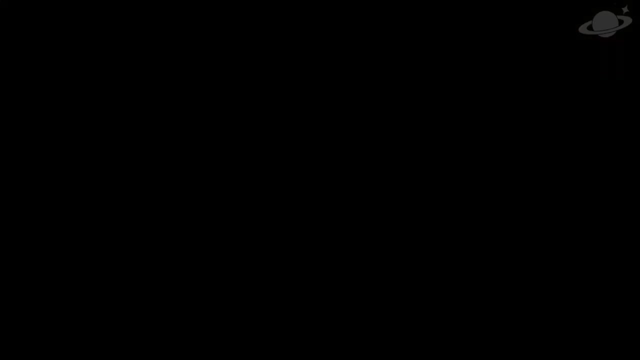 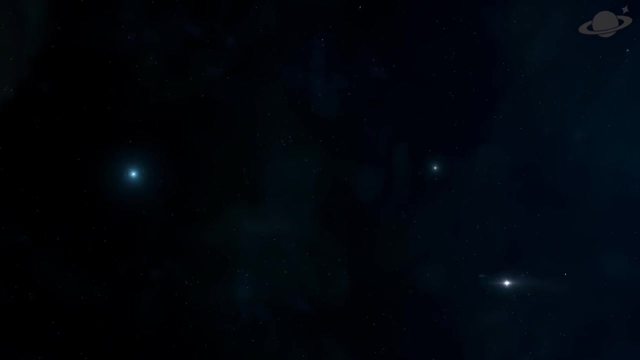 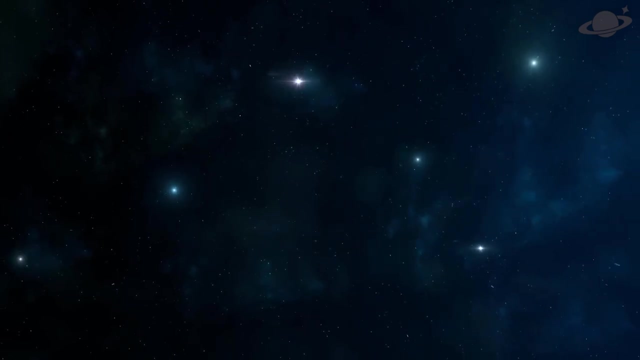 But because dark matter is so mysterious, we're still not sure about a lot of its properties and what it means for the universe's long-term future. Now let's look into thermodynamics a bit. Thermodynamics is a branch of physics. all about heat, temperature and how they're connected to energy and work. 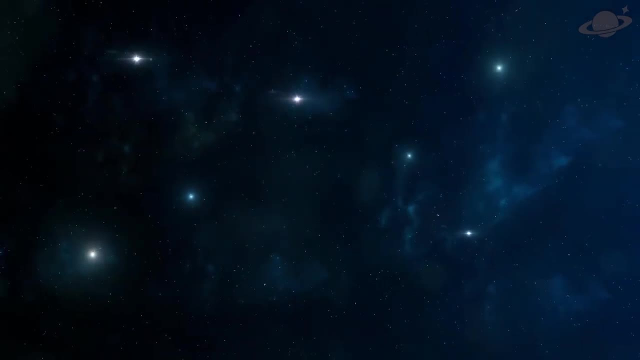 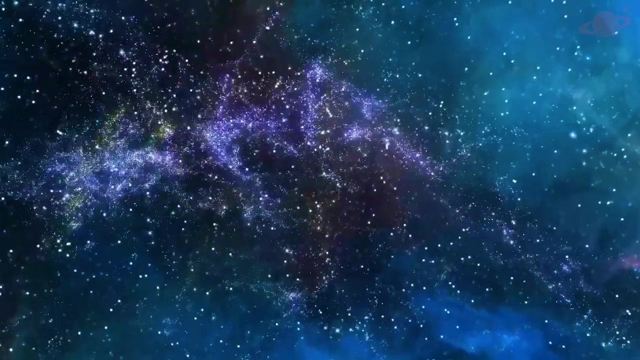 It's really important in figuring out what happens to the universe in the end. The laws of thermodynamics, especially the second law, are key to theories about how the universe will keep changing until it reaches its final state. The second law says that in a closed system, like the whole universe, 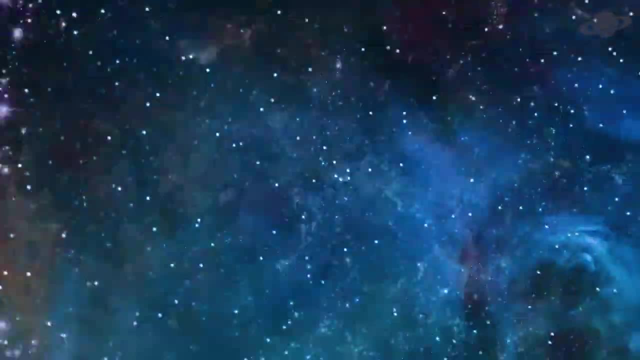 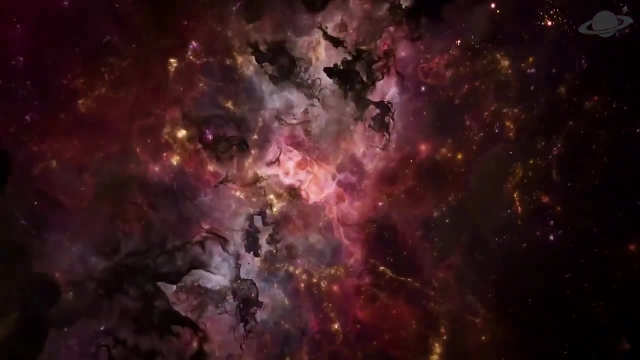 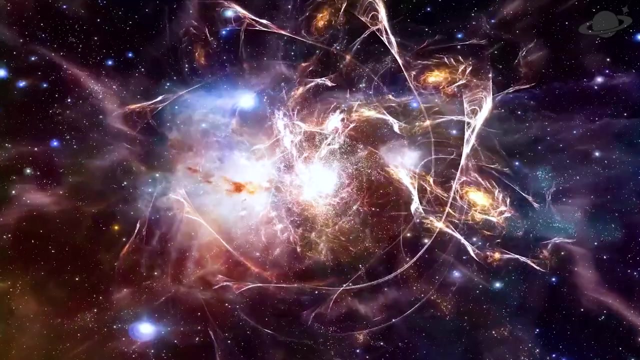 disorder, or randomness, always increases over time. Applying this to the universe means that its disorder keeps going up until it hits a maximum. This growing disorder has a big effect on what happens next. As disorder increases, the energy we can use to do things goes down. 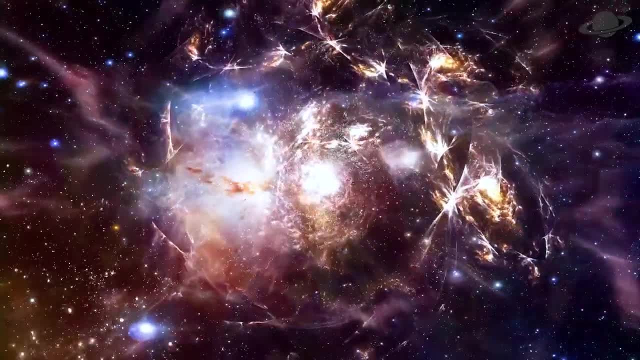 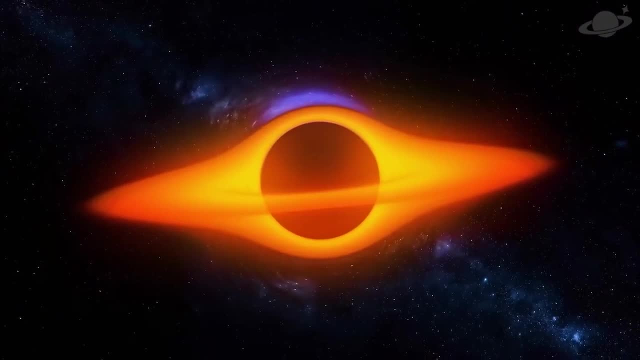 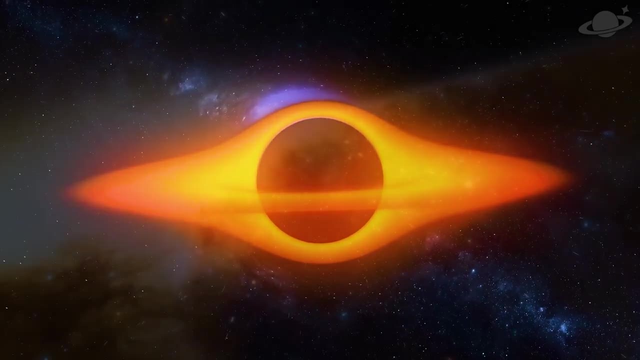 Until we reach a point where there's no more significant energy changes possible. We call this heat death or the big freeze. In this state, the universe hits a kind of energy balance, with energy spread out evenly everywhere and no more heat moving between different parts of the universe. 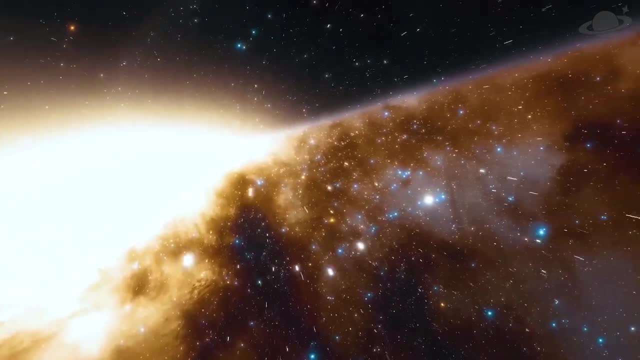 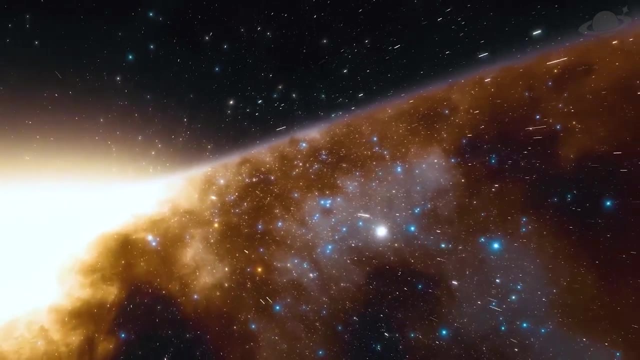 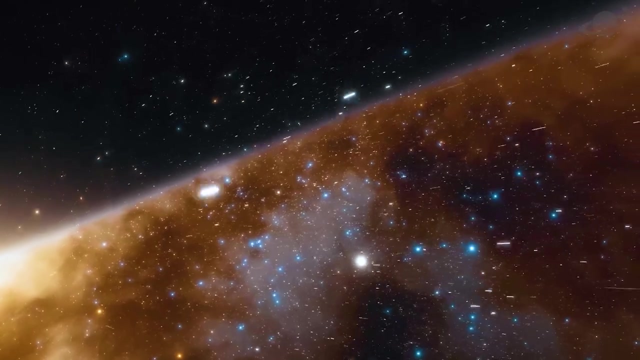 This even spread means that all processes relying on energy differences, like star burning, structure formation and even life, would stop. The idea of increasing disorder also links to how the universe expands. As the universe gets bigger, matter and energy spread out more, leading to more disorder. 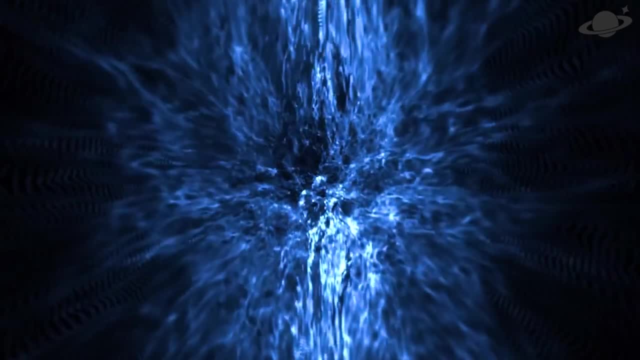 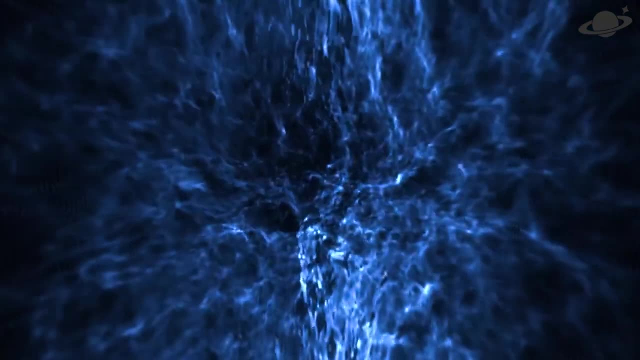 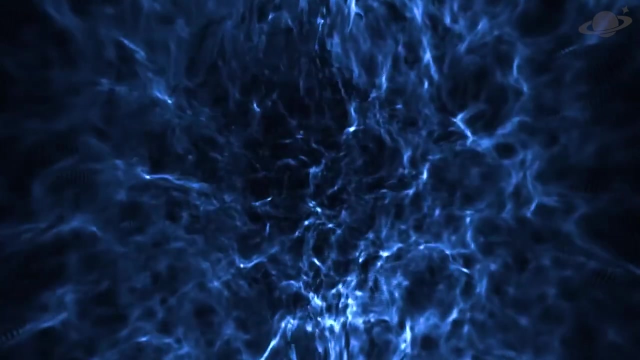 If the universe keeps expanding forever, as suggested by our current understanding of dark energy, this spreading out would keep increasing disorder, eventually leading to heat death. Additionally, the second law of thermodynamics might affect the flow of time. In our everyday experience, time moves in one direction, from past to future. 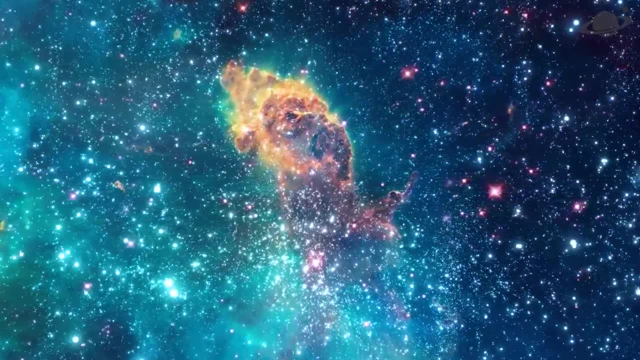 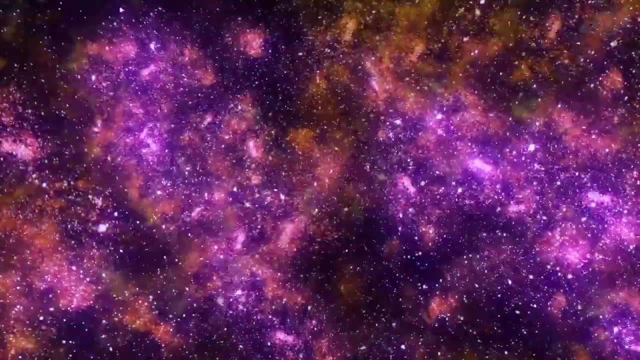 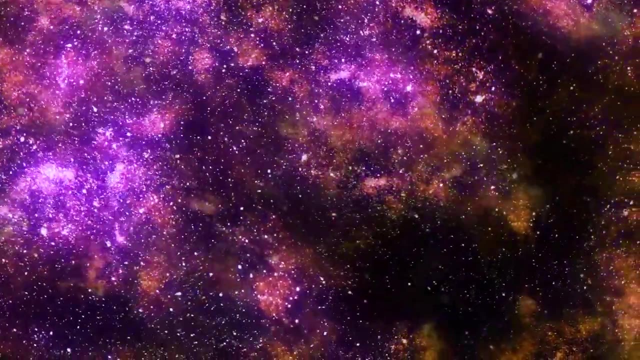 just like entropy increases. Some physicists think the growing disorder of the universe might be connected to how we see time moving. So if we know all this, what stops us from predicting how the universe will end? When trying to predict the universe's fate, our models run into several limits. 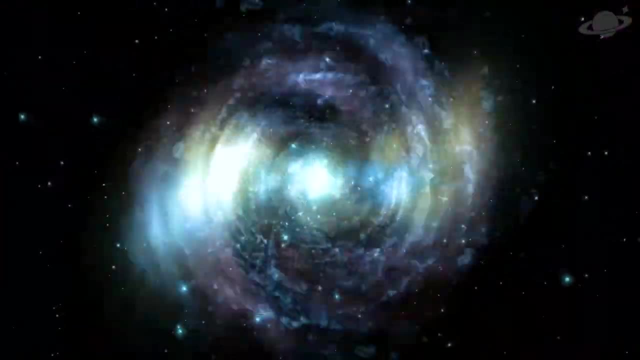 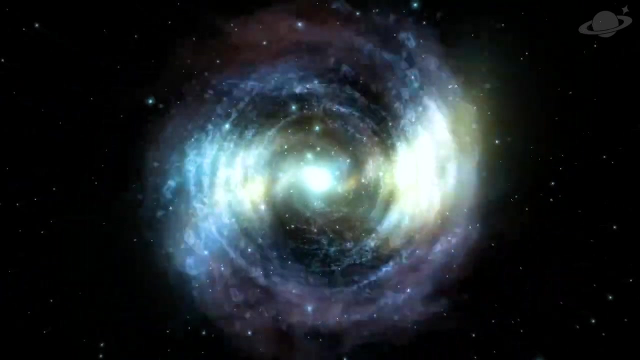 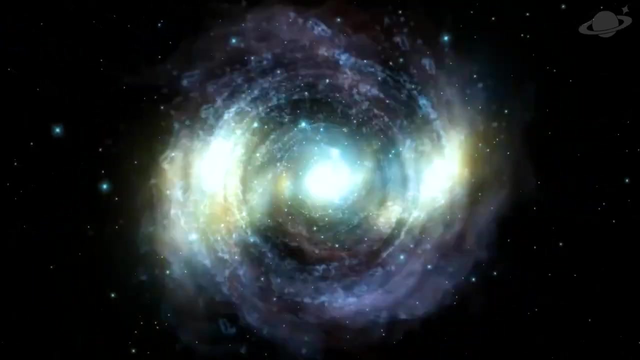 because of the huge complexity of space and our current scientific knowledge. These limits are crucial to recognize because they show where our understanding still needs work. One big limit is our limited grasp of dark energy and dark matter. These mysterious parts of the universe are key to how it changes, but we don't know much about them. 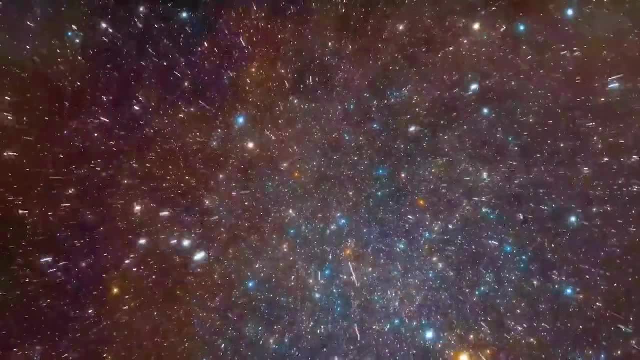 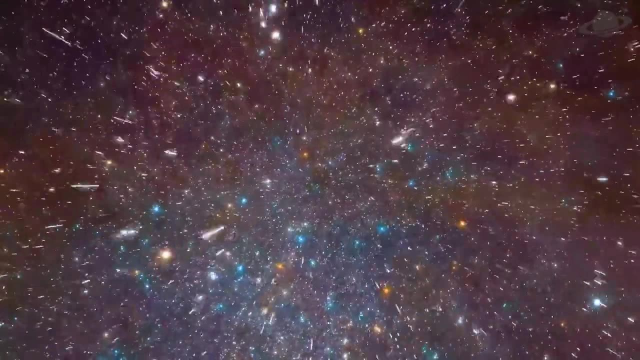 Dark energy, which speeds up the universe's expansion, can't be seen directly, and we figure out its properties from its gravity's effects. This means our models are missing some pieces, as we're working with an incomplete picture of what the universe is made of. 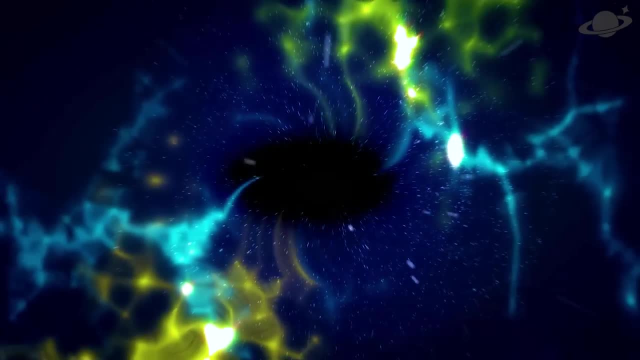 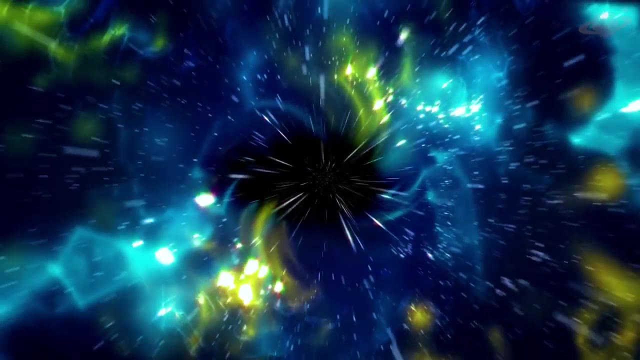 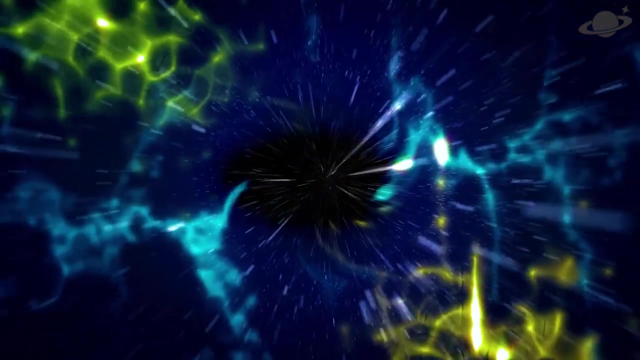 Another challenge comes from measuring distances and phenomena in space. The universe is incredibly huge and figuring out distances, speeds and other space stuff across such massive scales is really tough and can have mistakes, For instance, when we use things like Type YA supernovae as standard candles to measure distances. 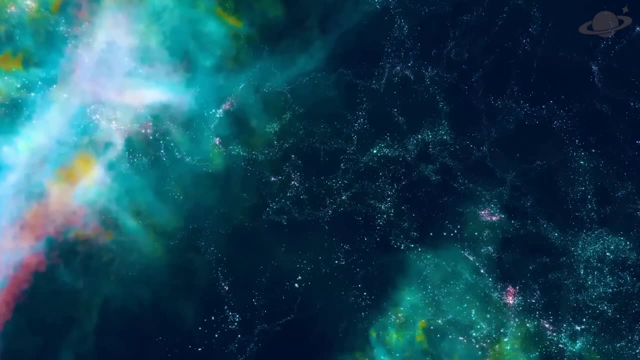 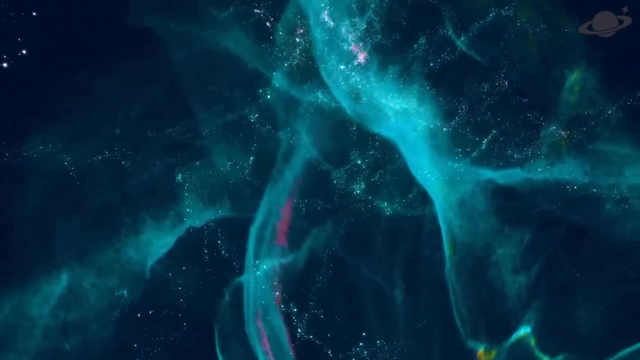 there's a whole bunch of steps involved, each with potential for mistakes. The Hubble tension is a big example of these measurement issues. It's about how we get different values for the Hubble constant, which shows how fast the universe is expanding. 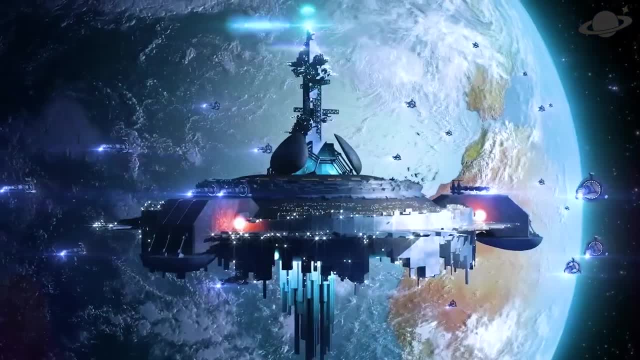 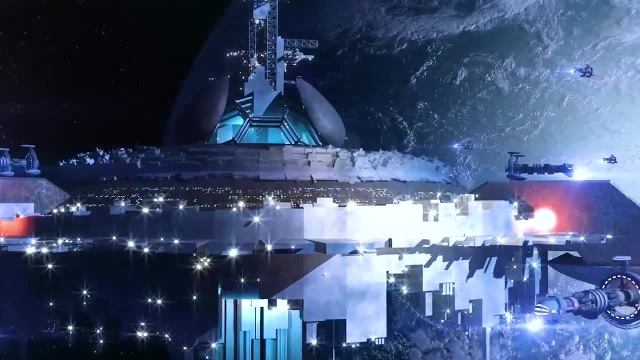 when we look at early universe stuff compared to stuff nearby. This difference suggests there might be things we don't know about affecting the universe's expansion, showing our models have limits. Also, our big theories like general relativity and quantum mechanics have their own limits. 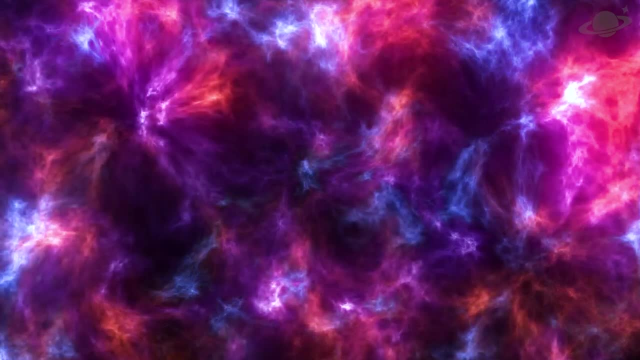 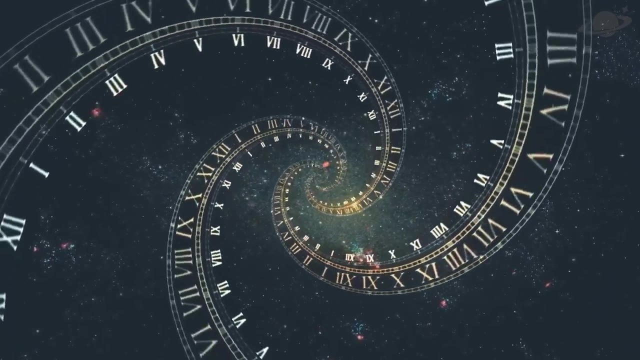 These are the basic ideas of physics, but they haven't been fully put together yet, especially in really extreme situations like black holes or the start of the universe. Since we don't have all the answers, our predictions might not be right in these extreme cases. 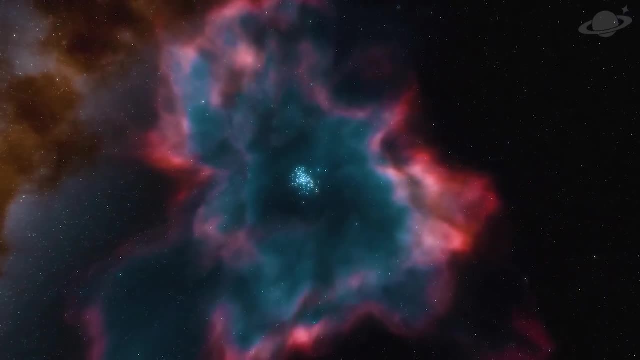 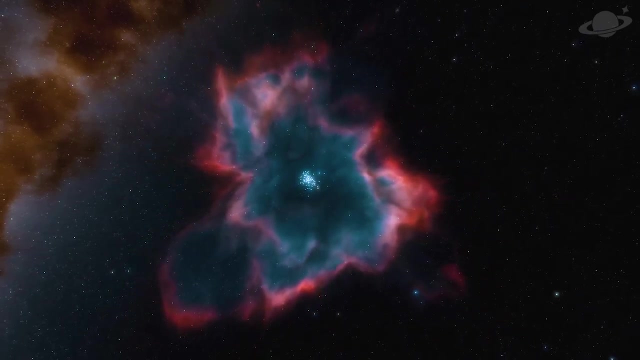 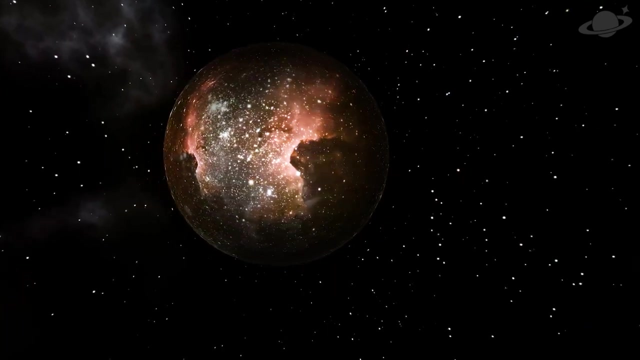 Lastly, science is always changing. What we know about the universe has changed a lot over time and will keep changing. New discoveries, better technology and new theories could totally change how we see the universe. How does entropy tie into the universe's end? Entropy, a concept from thermodynamics, is key to understanding how the universe works at different times. This data is super important for testing and refining ideas about the universe's future, like the Big Freeze or Big Rip scenarios. The CMB also tells us about the universe's shape and what it's made of. By looking at temperature and density differences in the CMB, astronomers calculate how curved the universe is and estimate how much ordinary matter, dark matter and dark energy there is. This helps us predict how these things will affect the universe's expansion and what might happen in the end. The discovery of the cosmic microwave background was a significant milestone in confirming the Big Bang theory, which forms the basis for many cosmological ideas about how the universe might eventually end. Essentially, the CMB tells us that the universe started out hot and dense. providing a crucial starting point for understanding its past and potential future. Studying the CMB in detail also helps to narrow down the possibilities for alternative theories about the universe's fate. Any viable theory must match up with what we observe in the CMB data. For example, theories suggesting a cyclic or oscillating universe, need to explain why the CMB appears uniform and has specific properties that we see today. As for whether we can simulate or model the universe's end, it's a challenging but active area of research for astrophysicists and cosmologists. They're using cutting-edge technology and complex math to try to understand and predict how the universe might evolve and eventually come to an end. To simulate the universe's end, scientists need to accurately model the various forces at work, including gravity, dark matter and dark energy. They do this by running sophisticated computer simulations that incorporate equations from general relativity. These simulations help visualize different scenarios, such as the Big Crunch, where the universe collapses back in on itself, or the Big Freeze, where it continues expanding indefinitely. For example, in simulations of the Big Crunch. researchers focus on how gravity might eventually overcome the expansion caused by dark energy. On the other hand, simulations of the Big Freeze project, the current rate of expansion into the future, considering how dark energy will continue to push galaxies apart until all activity stops. Furthermore, scientists use these models to delve into the mysteries. of dark matter and dark energy, two of the universe's most enigmatic components. By adjusting how these elements behave in their models, researchers can explore different outcomes and grasp how much the universe's fate hinges on them. While these simulations offer valuable insights, they're limited by our current grasp of the universe's laws and components. The accuracy of these models relies heavily on the data and theories they're built upon. For instance, any shifts in our understanding of dark energy or the discovery of new cosmic phenomena could significantly change the predicted results. Additionally, the immense time spans involved in cosmic evolution pose a challenge. These simulations often span billions to trillions of years, well beyond human lifetimes, making it hard to test and confirm predictions, keeping them largely in the realm of theoretical astrophysics. How does quantum mechanics affect our understanding of the universe's end? Quantum mechanics, the field of physics dealing with the tiniest particles, has profound implications for how we view the universe's ultimate fate. It introduces concepts that fundamentally alter scientists' perspectives on the cosmos, especially concerning its final state. One critical aspect where quantum mechanics plays a role is in the realm of black holes. Quantum theories like those involving Hawking radiation propose that black holes emit radiation and may gradually lose mass over immense periods. This concept suggests a mechanism by which even the most massive and long-lasting objects in the universe black holes could eventually vanish. In the context of the universe's end, this process could be significant, particularly in scenarios like the heat death, where black holes may be among the last structures remaining. Additionally, quantum mechanics introduces the idea of quantum fluctuations. small random changes in energy at a microscopic level. In a universe moving towards maximum disorder, as in the proposed heat death scenario, these fluctuations could have intriguing implications. Over unfathomably long periods, tiny fluctuations at the quantum level could potentially give rise. to new particle arrangements or even spawn entirely new universes, as some theories propose. This introduces a layer of unpredictability and complexity to our grasp of how the universe might eventually end. Another area where quantum mechanics plays a crucial role is in our investigation of dark matter and dark energy. Despite their critical role in shaping the universe's destiny, we still don't fully comprehend their nature. Quantum theories offer potential insights into the characteristics of these elusive components influencing our models of the universe's evolution, Furthermore, reconciling quantum mechanics with general relativity. stands as one of the greatest puzzles in modern physics. This reconciliation holds the key to understanding extreme cosmic conditions, such as those prevailing in the early universe or within black holes. Achieving this synthesis could profoundly alter our predictions regarding the universe's fate, particularly concerning scenarios involving cosmic collapse or rebirth. What role does time play in theories about the universe's end? Time occupies a central and fascinating position in our contemplation of the universe's ultimate fate. In simple terms, time measures the progression and change from one state to another. In cosmology, grasping the nature of time is crucial. for unravelling how the universe might unfold and eventually meet its end. Firstly, the vast temporal scales involved in these theories are mind-boggling. We're talking about billions to trillions of years into the future, surpassing all known human history or even the universe's current age. estimated at around 13.8 billion years. For example, the concept of the heat death of the universe, where all cosmic activity ceases due to maximum entropy, is projected to occur over a timeframe so immense that it dwarfs the discovery of new particles. religious beliefs and philosophical concepts. These cultural narratives often blend science, philosophy and spirituality, providing varied outlooks on the universe's ultimate fate. In Western traditions, heavily influenced by Judeo-Christian ideas, the end of the universe is often depicted as an apocalyptic event. 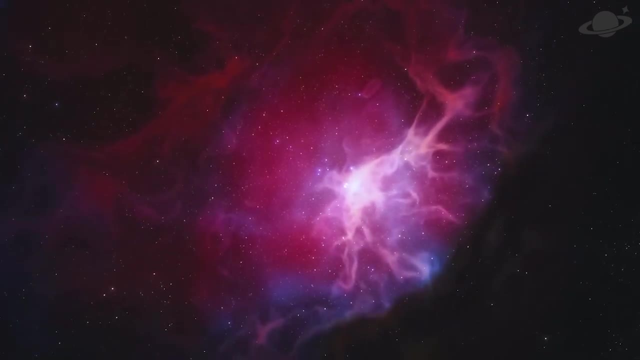 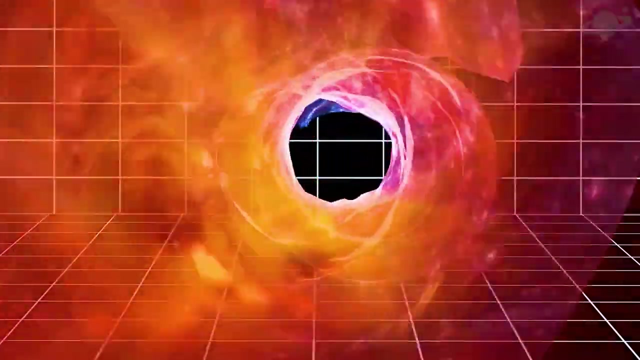 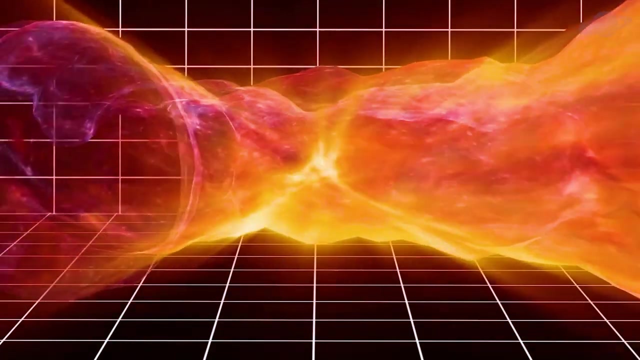 This perspective, found in texts like the Book of Revelation, portrays a final judgment and transformation rather than a literal end of the cosmos. It emphasizes moral and spiritual control over spiritual conclusions rather than scientific details. Conversely, many Eastern philosophies and religions, such as Hinduism and Buddhism, propose a cyclical view of the universe. 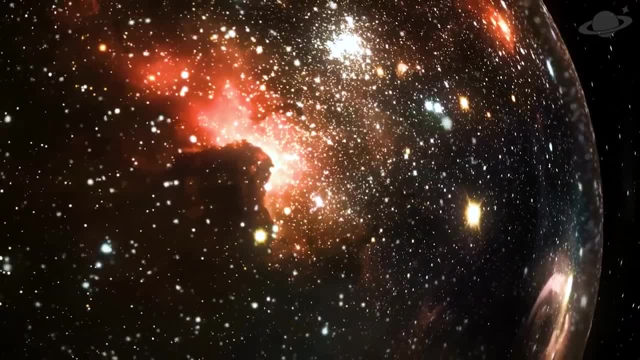 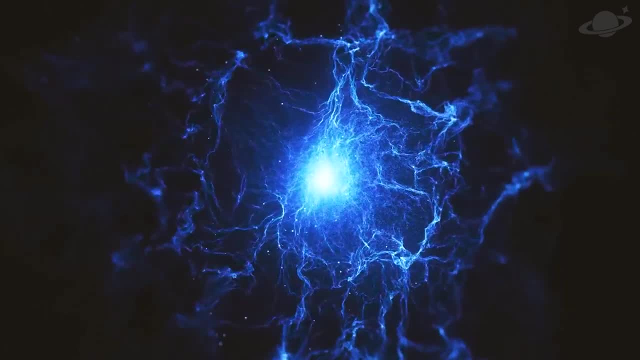 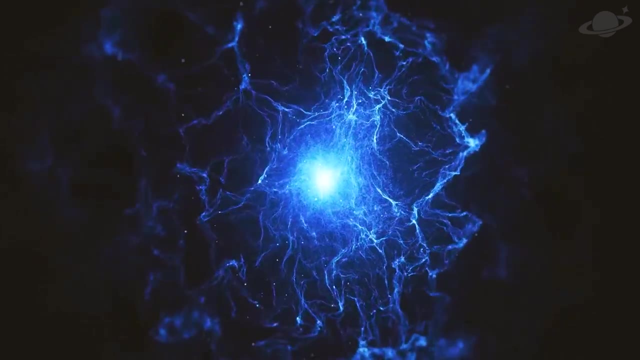 For example, in Hindu cosmology, the universe experiences repetitive cycles of creation, preservation and destruction, known as Mahayuga. This cyclic process holds not only physical significance, but also carries spiritual meaning, symbolizing the eternal rhythms of birth, life and rebirth. 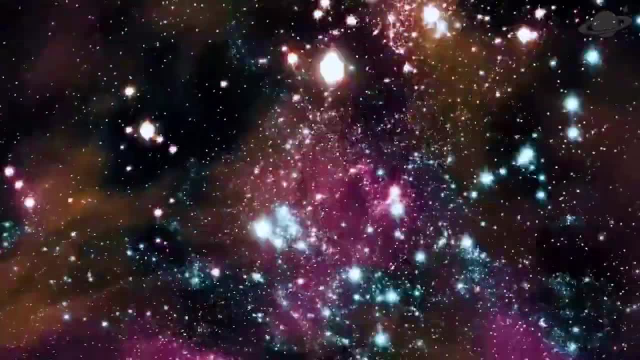 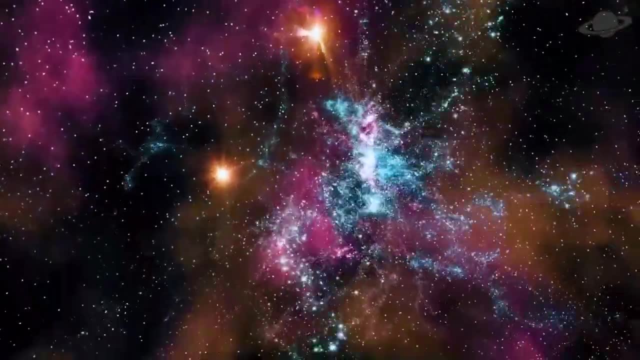 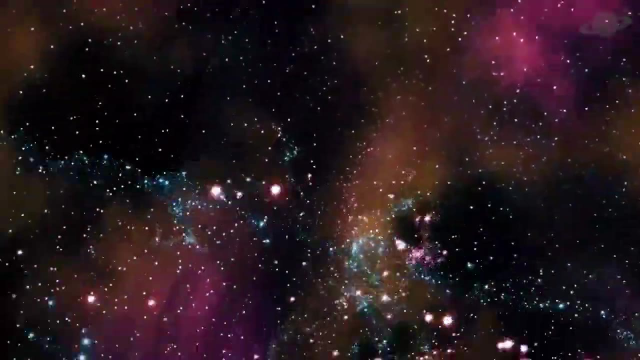 Indigenous cultures across the globe also offer their own interpretations. Some Native American traditions, for instance, speak of a sequence of worlds or ages, each concluding with a transition to the next through various forms of renewal or destruction. These stories often highlight the importance 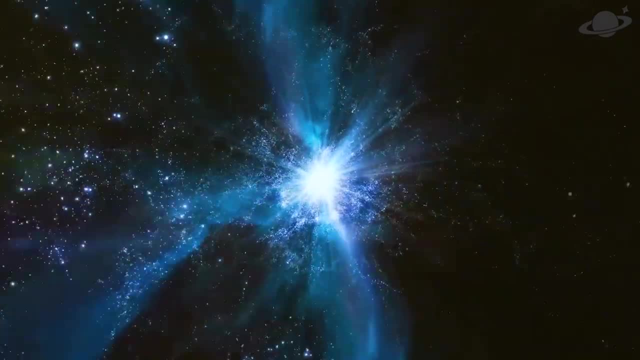 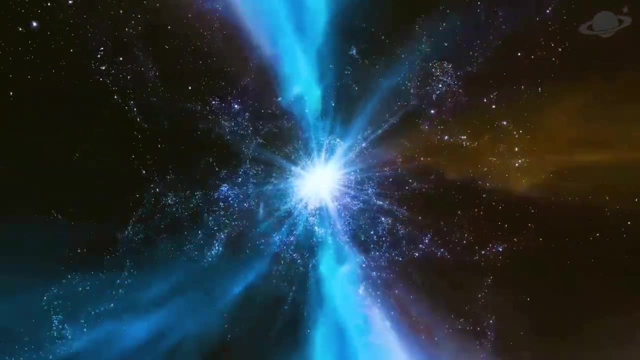 of living in harmony with nature and recognizing the interconnectedness of all living beings, portraying the end of the universe as a natural and sacred part of a larger cycle. For instance, in Norse mythology there's the concept of Ragnarok, a series of events that include a great battle. 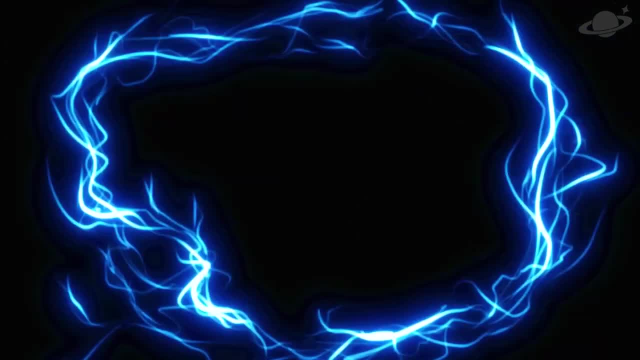 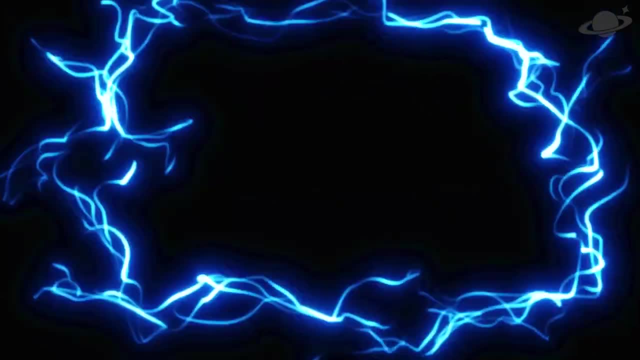 resulting in the death of major gods and a world flood. After these cataclysms, it's prophesied that the world will emerge anew and fertile, with surviving gods reuniting and two humans repopulating the earth In modern times. 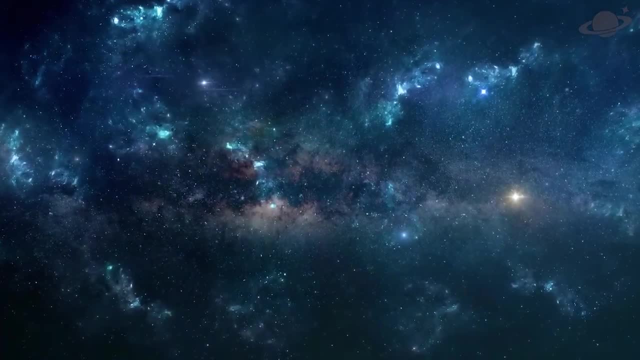 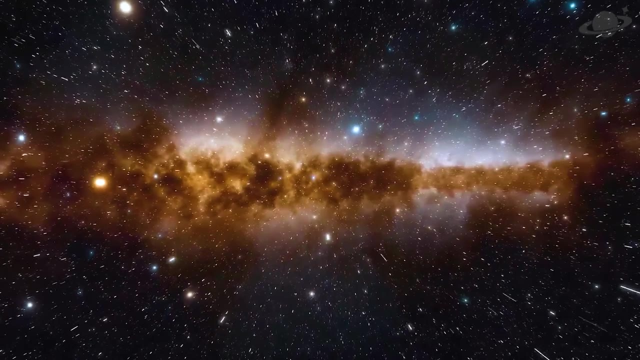 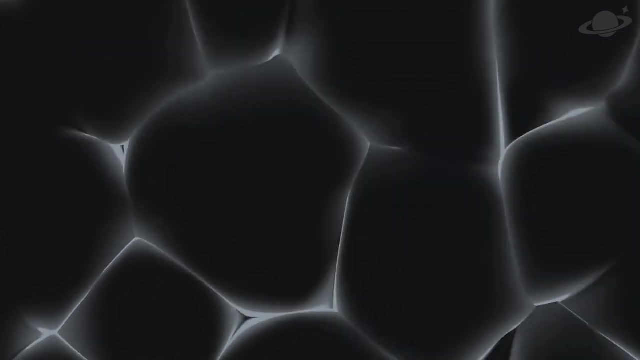 as our scientific understanding of the universe has grown, these cultural tales have sometimes intertwined with scientific theories. For example, the notion of an expanding universe heading towards a cold, dark end may resonate with both apocalyptic and cyclical beliefs, seen as either the final state of entropy or just one phase. 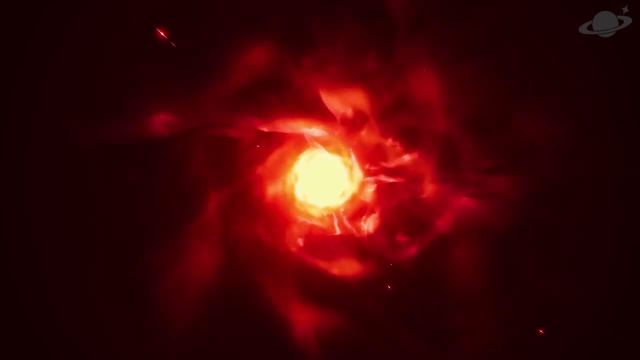 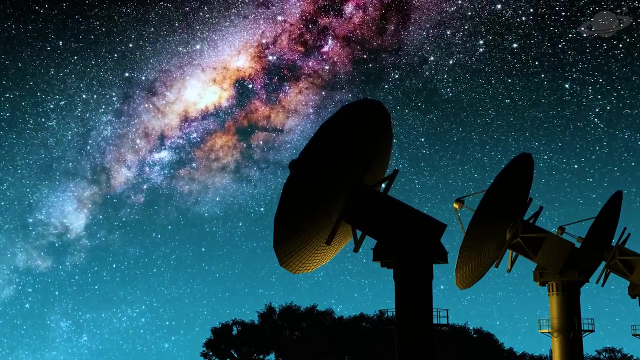 in an ongoing cycle of cosmic events. Each of these cultural viewpoints not only reflects ideas about the end of the universe, but also deeper values and insights about life, existence and the nature of change and continuity. They show how humans have long pondered. 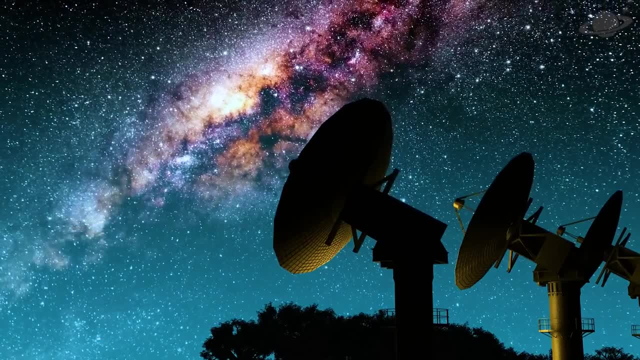 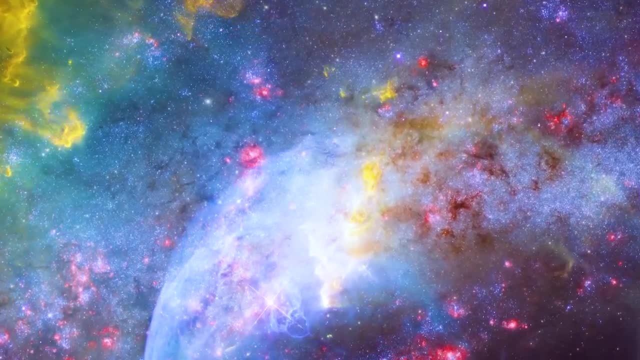 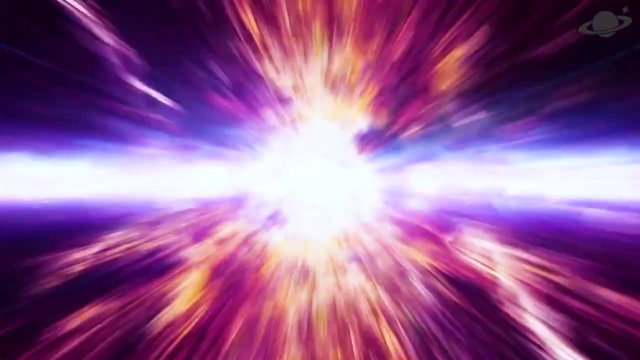 not only the physical aspects of the cosmos, but also its metaphysical and spiritual dimensions, from its beginning to its end. Now let's delve into an intriguing hypothesis. The vacuum decay hypothesis is a captivating and somewhat unsettling idea in the realms of cosmology and theoretical physics. 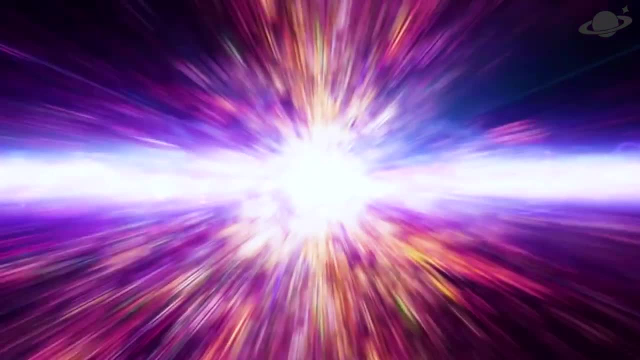 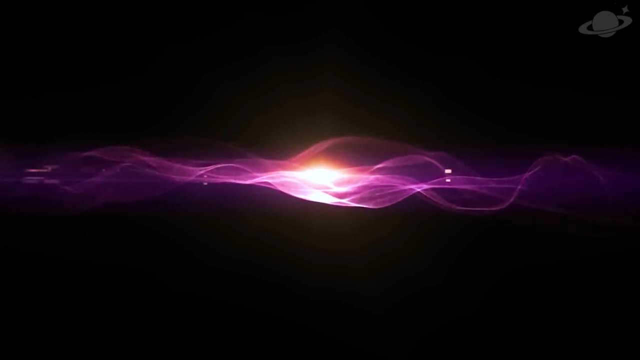 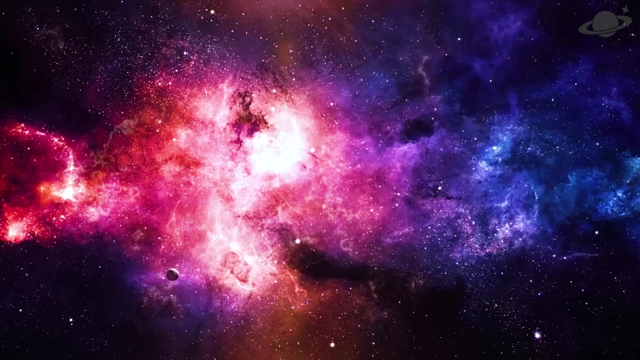 It proposes a scenario where the universe doesn't end with a bang or a whimper, but with a bubble. This hypothesis revolves around the notion of a false vacuum, a tentative or unstable state of space containing potential energy. In this scenario, our current universe exists in a false vacuum. 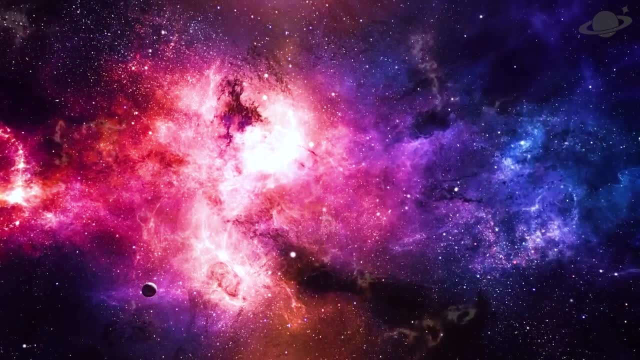 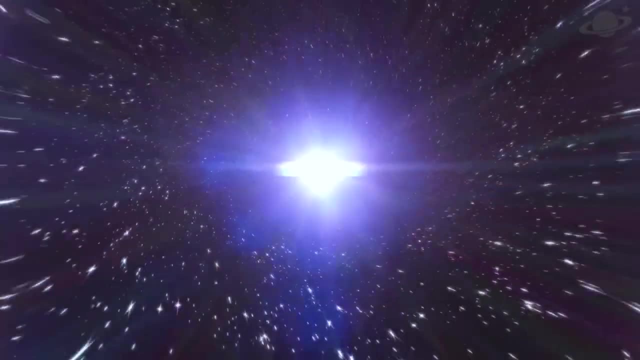 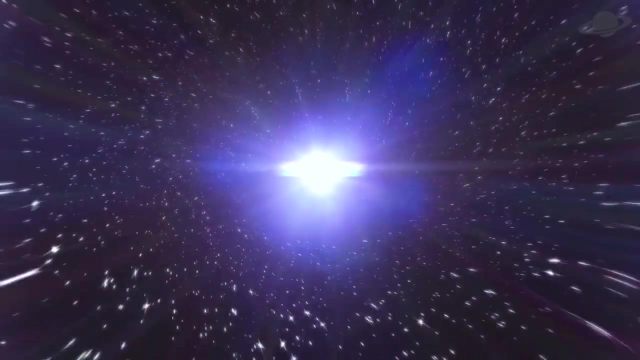 a temporary and unstable condition that could decay into a more stable state, known as the true vacuum. This decay could be triggered by a random quantum fluctuation creating a bubble of this true vacuum. What's particularly unsettling about this hypothesis is what happens next. 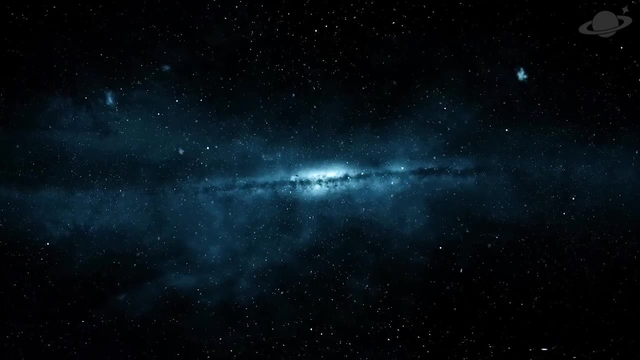 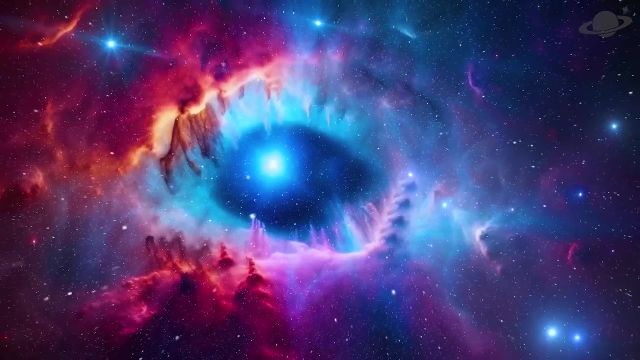 This bubble would expand at the speed of light, altering anything it touches. at a fundamental level, The laws of physics as we know them might completely change inside this bubble, Everything we're familiar with: galaxies, stars, planets and even the basic components of matter. 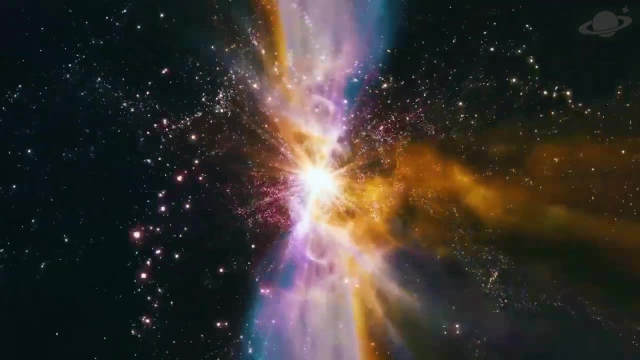 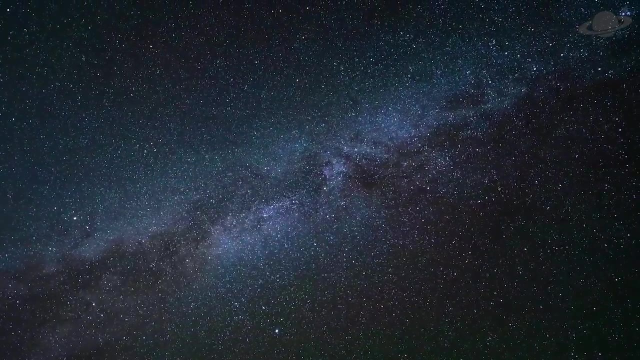 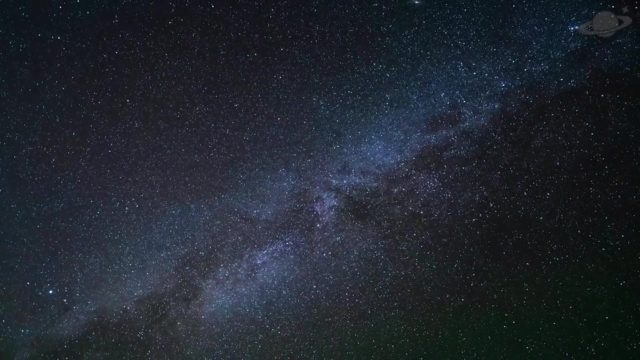 could be destroyed or drastically transformed as the bubble engulfs them. The vacuum decay theory is purely theoretical and not something we can expect to happen anytime soon. It's based on ideas from quantum mechanics and quantum field theory, which study how the universe behaves at its smallest levels. 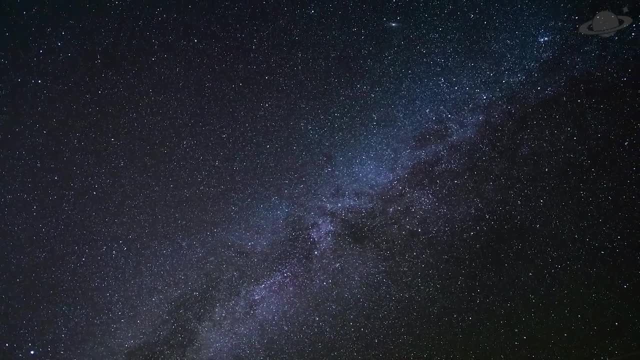 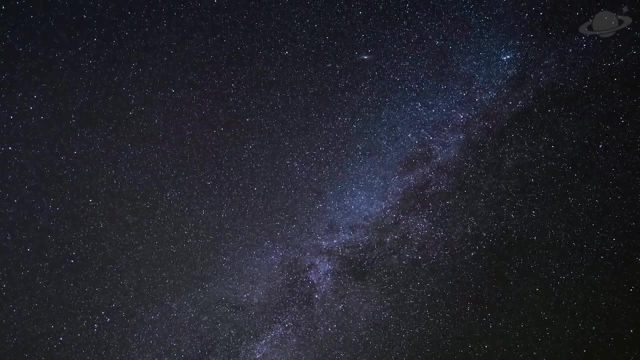 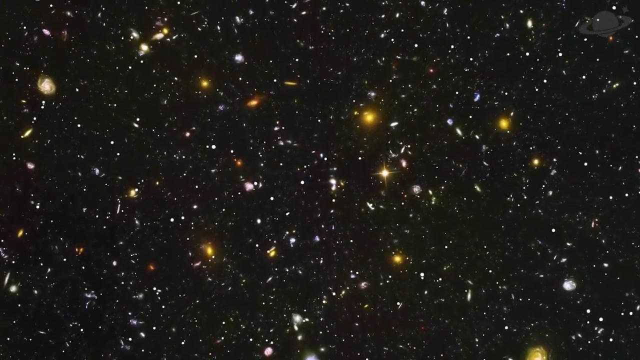 The theory suggests that what we think of as empty space might actually be filled with invisible energy fields. One interesting aspect is that this process could occur suddenly and without warning, because it would spread at the speed of light. We wouldn't see it coming, But it's important to understand that this theory 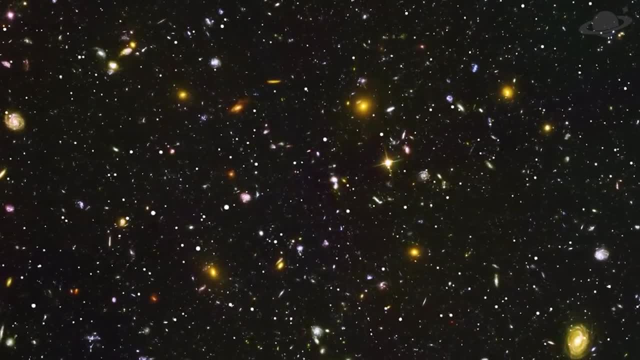 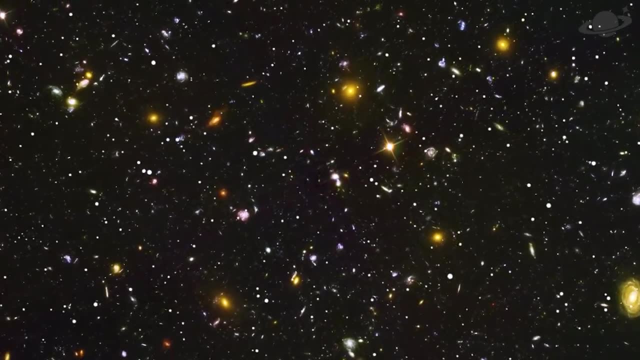 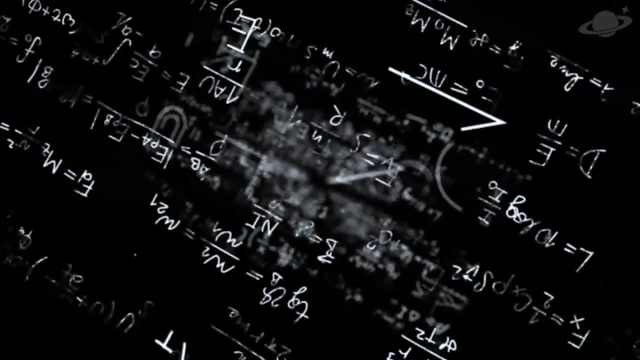 is just one of many speculative ideas about how the universe might eventually end. Can advancements in technology help us understand the universe's end better? Absolutely, Technological progress has always been crucial in expanding our knowledge of the cosmos, and it's key to uncovering new insights. 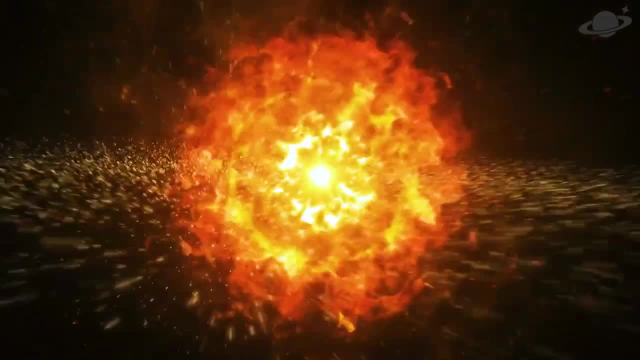 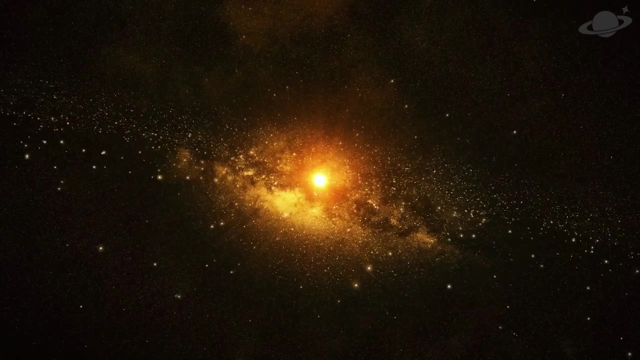 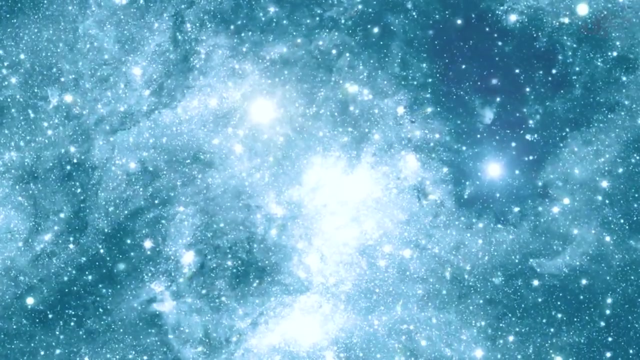 into how the universe might meet its end. As we develop better tools and computer models, our ability to observe, measure and understand cosmic events improves, bringing us closer to answering some of the universe's biggest questions- One area where technology is making a big difference. 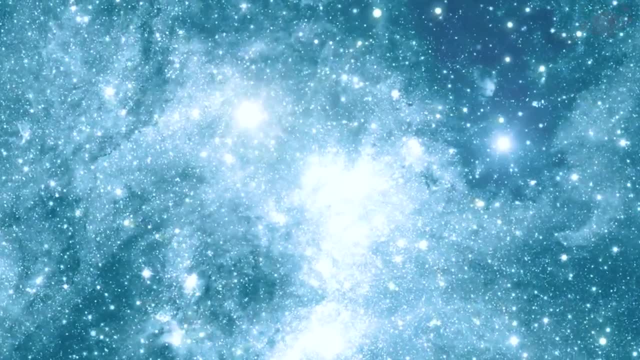 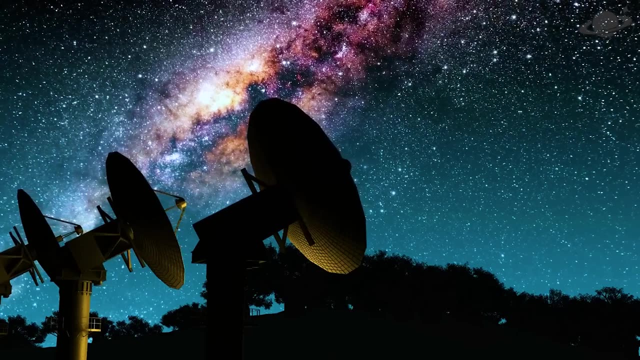 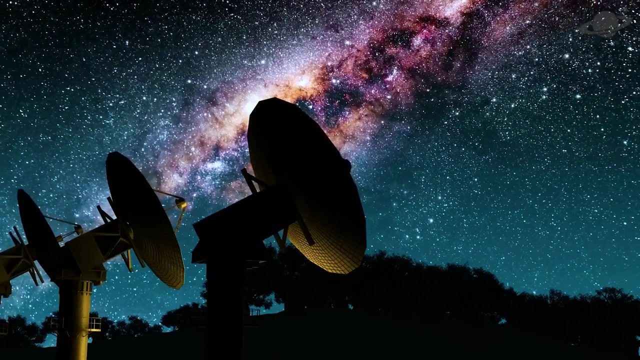 is in observational astronomy. New telescopes, both on the ground and in space, allow astronomers to see distant cosmic phenomena more clearly than ever before. For example, telescopes like the James Webb Space Telescope can peer deeper into space, potentially revealing new information about the early universe. 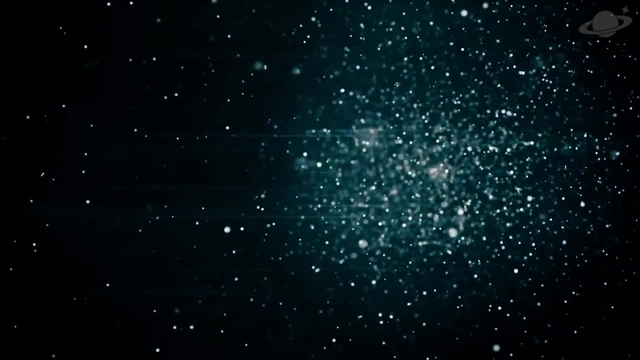 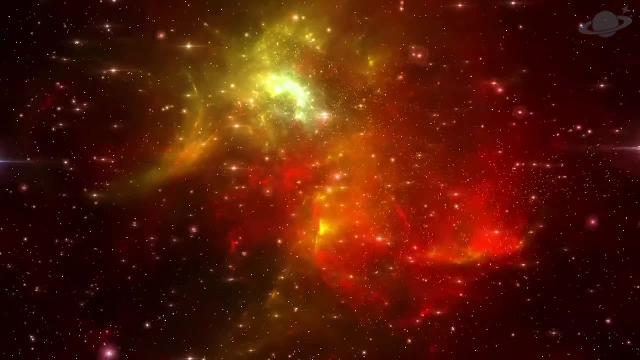 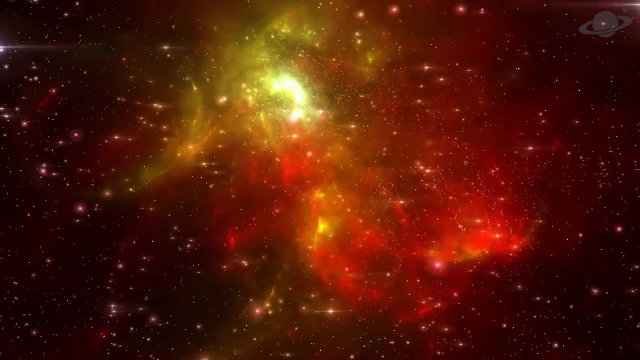 that could help us predict its end. Alongside observational tools, advances in computing are also crucial. Supercomputers can now process vast amounts of data and run complex simulations faster than ever. These simulations let scientists model different scenarios for the universe's end. 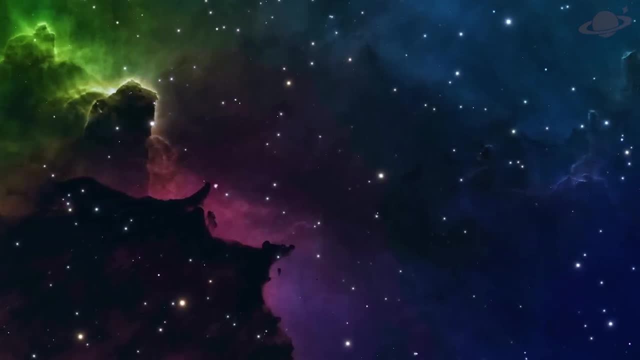 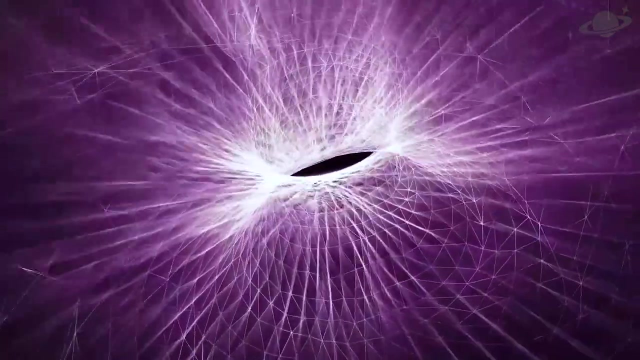 from the Big Freeze to the Big Rip with incredible detail. By tweaking variables in these models, researchers can explore a wide range of possible outcomes. Furthermore, progress in particle physics, aided by technologies like particle accelerators and detectors, helps us understand the fundamental forces. 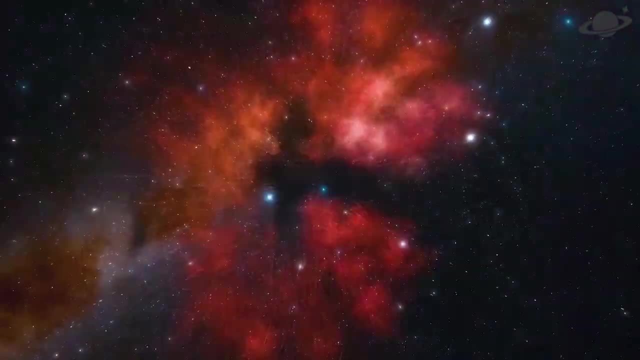 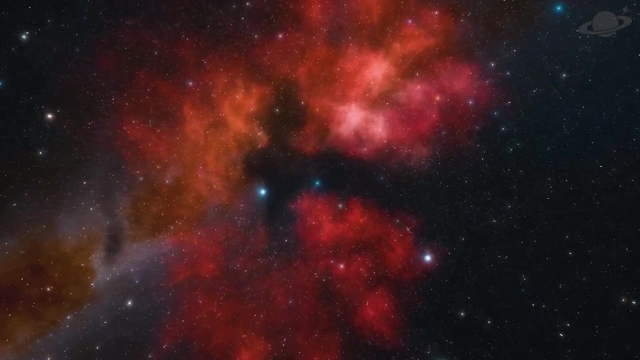 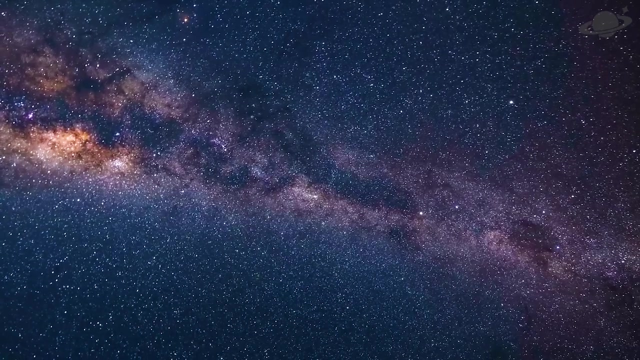 and particles shaping the universe's behavior. Discoveries in this area could help us understand dark matter and dark energy, two crucial factors shaping the fate of the universe. For example, experiments at places like the Large Hadron Collider, LHC, might reveal new particles or phenomena. 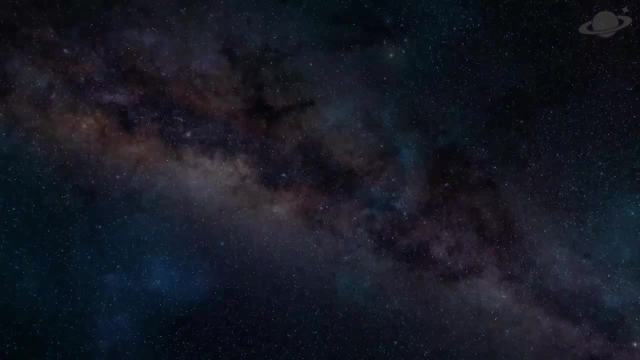 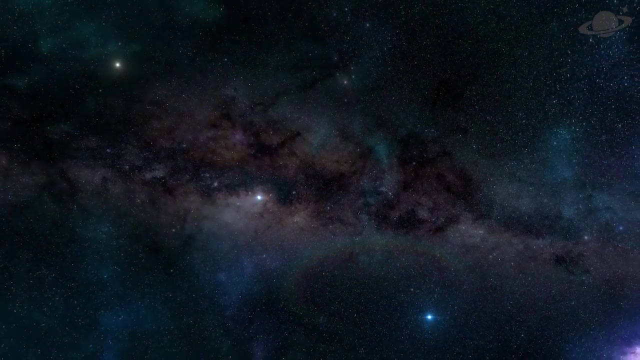 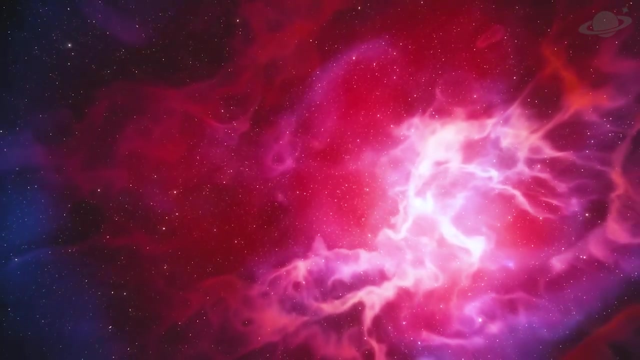 that could change our view of the cosmos. Advancements in fields like quantum computing and nanotechnology could also offer hope for cosmological research. Quantum computers, for instance, could tackle complex problems and analyze data in ways we can't do currently, potentially offering fresh insights into the quantum side. of the universe and its eventual destiny. Supernovae are another fascinating aspect of studying the universe's end. These explosive events mark the finale of a star's life and are vital for understanding cosmic conclusions and the wider story of the universe. They aren't just visually spectacular. they're also treasure troves of information, helping astronomers unlock secrets of the cosmos, including hints about its eventual fate. When a star goes supernova, it shines brighter than entire galaxies for a brief period, emitting huge amounts of light and energy. This makes supernovae visible across vast distances. turning them into important markers in cosmic exploration. One of their significant roles is as standard candles. Certain types, like Type Ia supernovae, always reach a consistent brightness at their peak, allowing astronomers to accurately measure their distance from Earth By gauging the distance to these supernovae and their redshift. how fast they're moving away from us due to the universe's expansion. scientists can work out the rate of this expansion. This method led to a groundbreaking discovery: that the universe's expansion is actually speeding up. This finding led to the theory of dark energy, a mysterious force propelling this acceleration. Studying supernovae is like unlocking a cosmic treasure trove with profound implications for our understanding of the universe's destiny. These colossal explosions not only mark the dramatic end of stars, but also offer clues about the fate awaiting our cosmos. They shed light on the mysterious force known as dark energy. which holds the key to how the universe might end, whether it's in a big freeze, big rip or another scenario. Additionally, supernovae have a crucial role in the cosmic recycling of matter. When they explode, they scatter heavy elements across space. which are vital for creating new stars in the long run. Additionally, the large-scale layout of the universe can help us understand its overall shape and structure, which is vital in predicting what might happen to it in the future. If the universe is closed, it could eventually stop expanding. and start to collapse in on itself, leading to a potential scenario known as the Big Crunch. On the other hand, if it's open or flat, which is what current evidence suggests, it will likely keep expanding forever, possibly resulting in a big freeze or big rip. The way cosmic structures are spread out also has implications for how energy is distributed and how disorder entropy increases over time, which is crucial in theories like the heat death. As the universe changes over time, energy becomes more spread out across its vast expanse. The way the universe is structured affects how this spreading happens and how disorder increases over time, which is a big part of theories like the heat death. What role does string theory play in understanding how the universe will end? String theory, a field of physics that tries to bring together quantum mechanics. and general relativity offers a unique view on how the universe might end. It suggests that, instead of tiny point-like particles, the fundamental building blocks of the universe are tiny vibrating strings. While string theory is quite complicated and mostly speculative, it introduces ideas that could change how we see the universe and its future. One fascinating idea in string theory is that there could be more than just the three dimensions of space and one of time that we are familiar with. These extra dimensions could have a big impact on how the universe evolves over time. For example, how these dimensions change over time might affect how fast the universe expands. or even the nature of darkness. String theory also explores quantum gravity, which is a field aiming to describe gravity using the principles of quantum mechanics. Understanding quantum gravity is crucial for explaining phenomena such as black hole, singularities or the conditions during the early universe. When considering the end of the universe. a better grasp of quantum gravity could offer insights into how the universe might behave as it keeps expanding, potentially uncovering new scenarios beyond those currently favored, like the Big Freeze or the Big Rip. Furthermore, string theory introduces the idea of multiple universes or a multiverse. This notion suggests that our universe might be just one of many, each possibly governed by different physical laws. If this aspect of string theory proves true, it could profoundly change our understanding of the universe's fate. Our universe's destiny might only be a part of a much larger and more complex multiverse. where each universe has its own distinct end. What are the signs that indicate the universe is moving towards its end? Detecting these signs involves a blend of intricate astronomical measurements and theoretical predictions, While the end of the universe is a far-off event, projected to happen over an immensely long timescale. there are observable phenomena that offer clues about its eventual winding down. One significant sign is the rate at which the universe expands. Astronomers measure this expansion by observing the redshift of distant galaxies, how their light stretches to longer, redder wavelengths as they move away from us. This redshift confirms not only that the universe is expanding, but also helps scientists determine how fast this expansion is occurring. The discovery of the universe's accelerating expansion was a crucial moment in cosmology, indicating the influence of dark energy If this acceleration persists. it supports scenarios like the Big Freeze, where the universe would continue expanding indefinitely, becoming colder and emptier over time. Another indicator is the life cycle of stars. Stars are like the universe's power plants and by studying how they are born, live and die. astronomers can learn a lot about what the universe might look like in the distant future. As the universe gets older, the rate at which new stars are formed is expected to slow down, and the stars that already exist will gradually run out of fuel. By looking at galaxies that are older and where star formation has slowed down a lot, we can get an idea of what might happen to our own galaxy billions of years from now. The behavior of galaxies themselves also gives us hints about the universe's future. In a universe that's heading towards a cold and isolated end, we'd expect to see galaxies moving away from each other more and more over time. This means that the rate of galaxies crashing into each other and merging would also slow down. Telescopes that are very powerful can observe these movements and interactions, providing data that fits into our long-term models of what might happen to the universe. Furthermore, the fate of the universe is connected to the way cosmic structures like black holes behave. 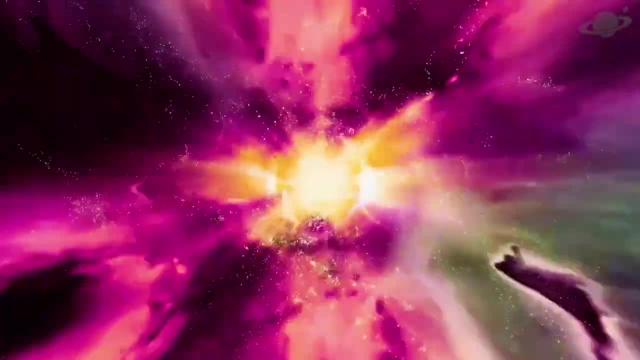 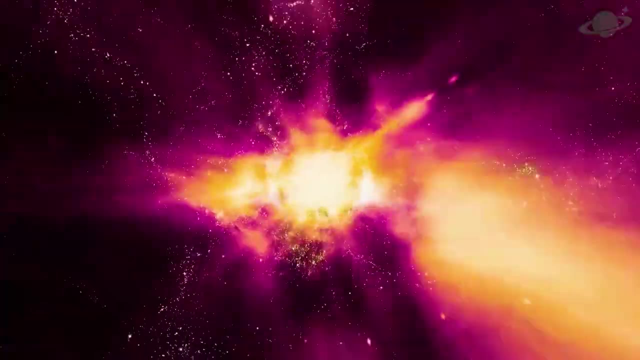 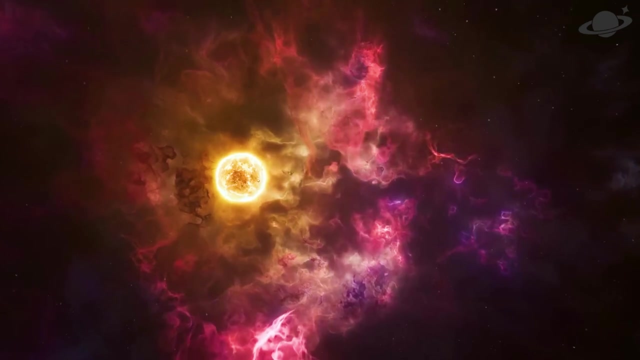 According to theories like Hawking radiation black holes should emit radiation very slowly, which means they would gradually evaporate over incredibly long distances. This gives us an idea of what might happen to our own galaxy billions of years from now. By studying black holes and their properties, gives us insight into these far-off events. 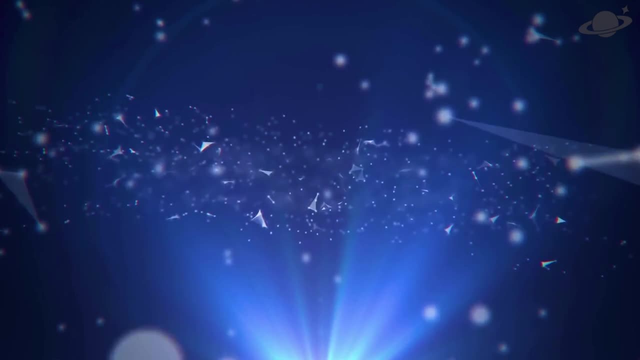 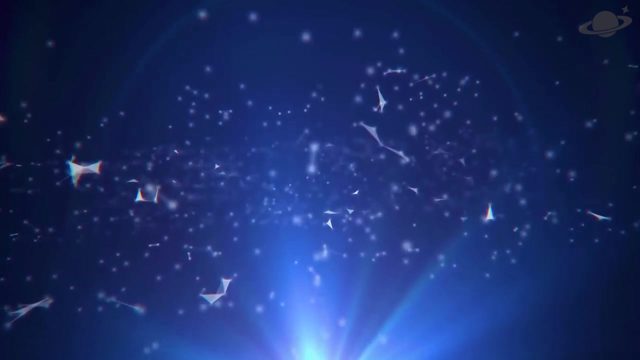 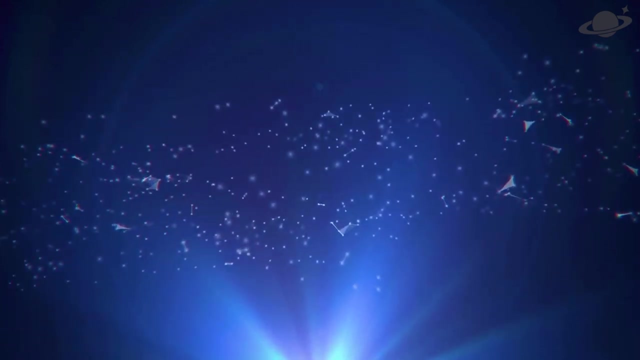 From black holes to light. how does the speed of light affect how we see the universe's end? The speed of light is crucial in how we observe and understand what might happen to the universe in the future. Light travels incredibly fast, at about 299,792 km per second. 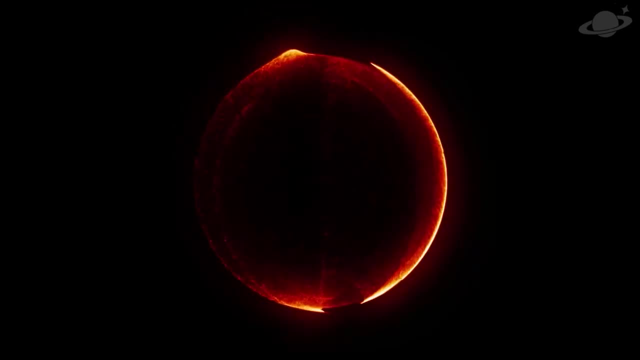 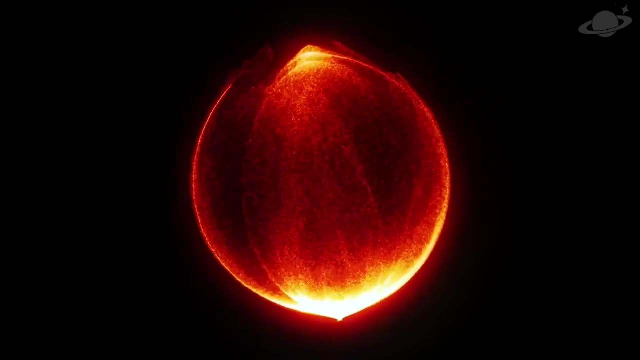 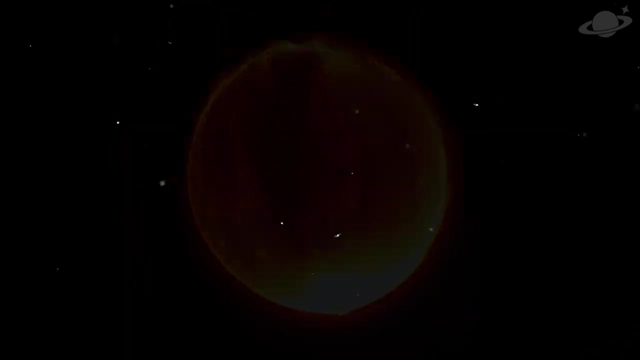 and this finite speed influences how we perceive the universe in important ways. The speed of light sets a boundary on how far we can see into the universe and consequently, how much we can learn about its destiny. When we observe distant objects in space, we're essentially peering back in time. 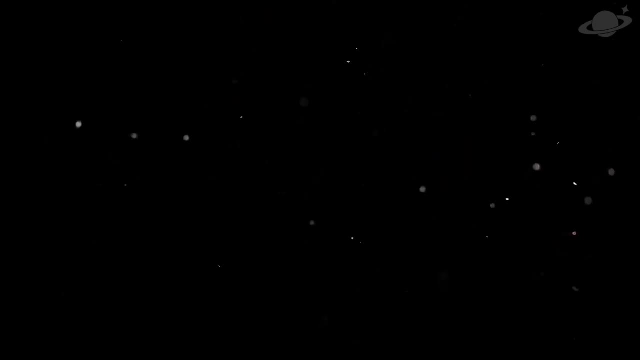 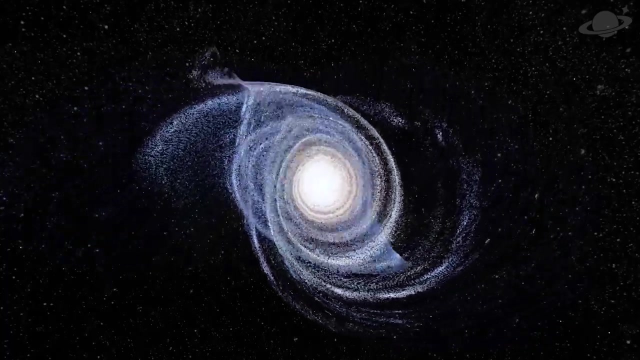 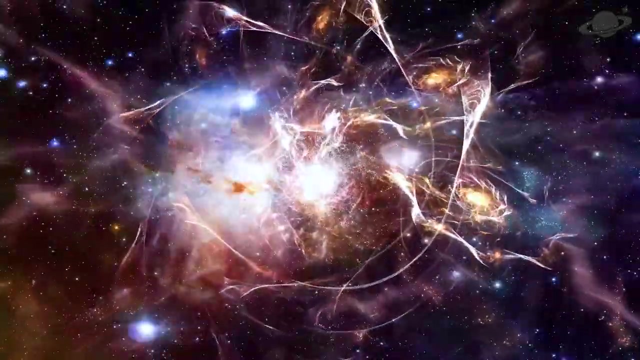 For instance, if we see a galaxy that's one million light-years away, we're seeing it as it was one million years ago, because that's how long it took for the light from that galaxy to reach us. This concept, known as look-back time, allows astronomers to study how the universe has changed over time. 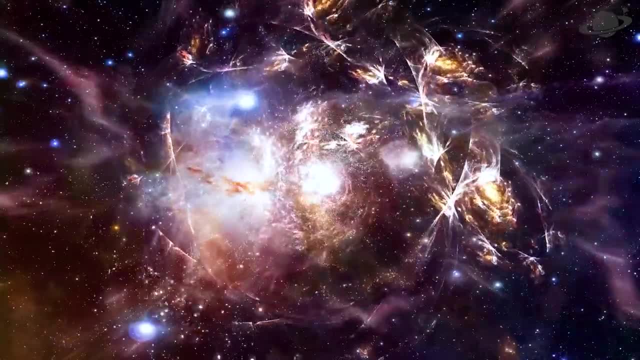 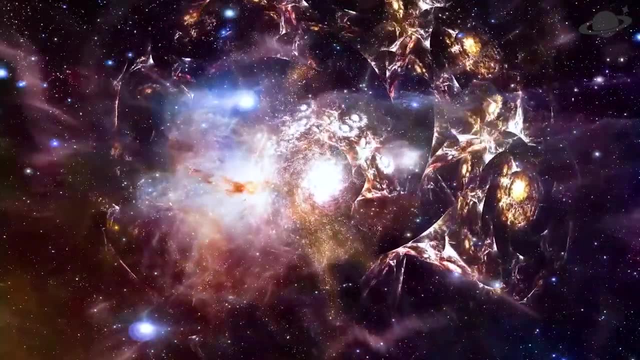 By observing galaxies at different distances, we can construct a timeline of the universe's expansion and make predictions about its future. However, there's a limit to how far back we can look. The cosmic microwave background radiation, which is the afterglow of the Big Bang. 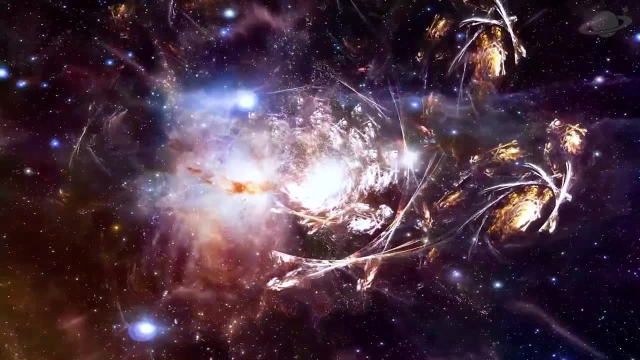 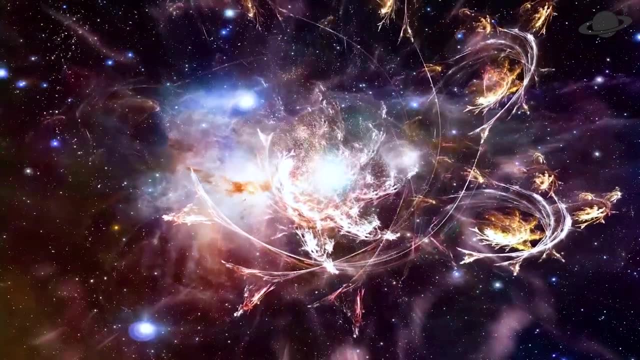 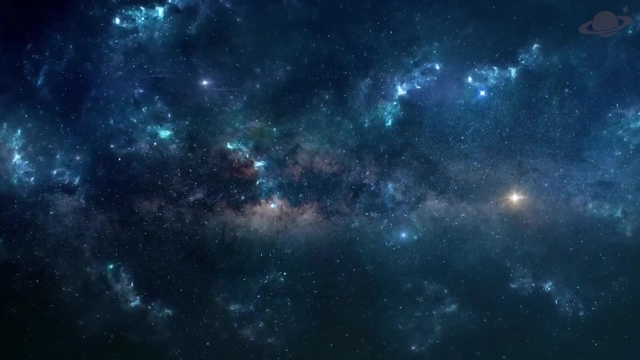 is the oldest light we can detect, dating back to about 380,000 years after the universe began. Before this point, the universe was opaque to light, which means we can't directly see its earliest moments. This limitation also means there's a cap on our direct knowledge of the universe's future. 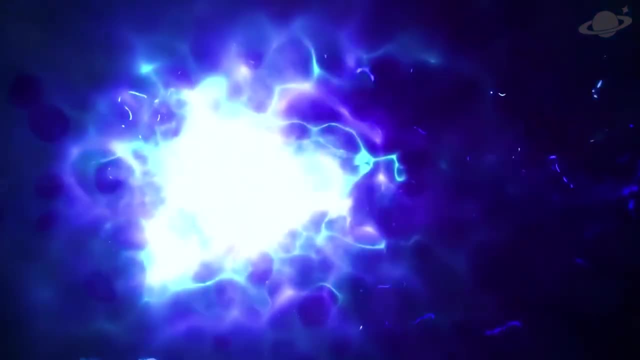 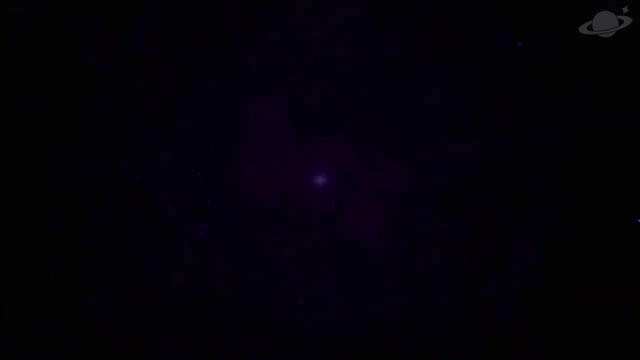 since we can only infer what lies beyond based on our current understanding of physics In terms of the universe's eventual end. the speed of light means that any observable changes, such as the accelerated expansion caused by dark energy, are seen with a delay. 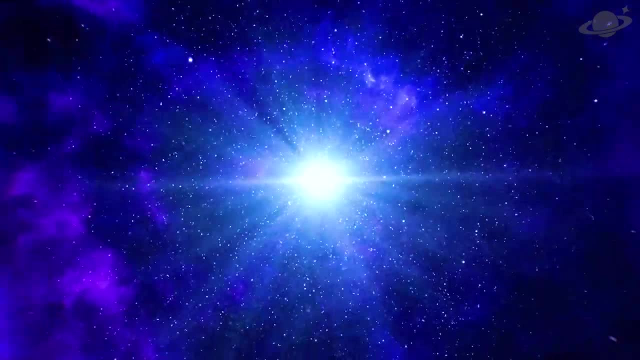 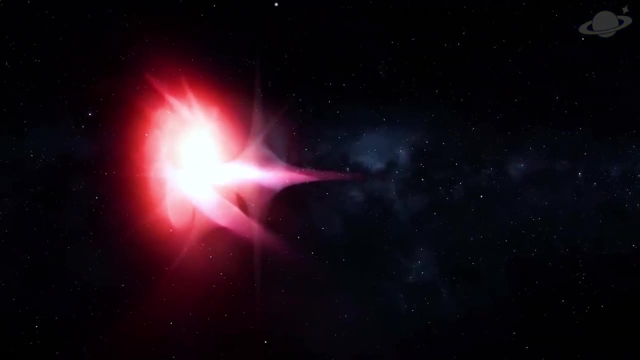 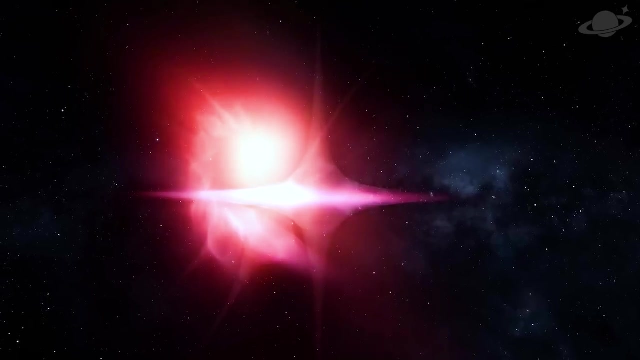 If the universe were heading towards a scenario like the Big Bang or the Big Rip, where galaxies, stars and even atoms are torn apart by the rapid expansion of space, we wouldn't witness these events until long after they've happened. The speed of light also affects our comprehension of events that might signal the universe's end. 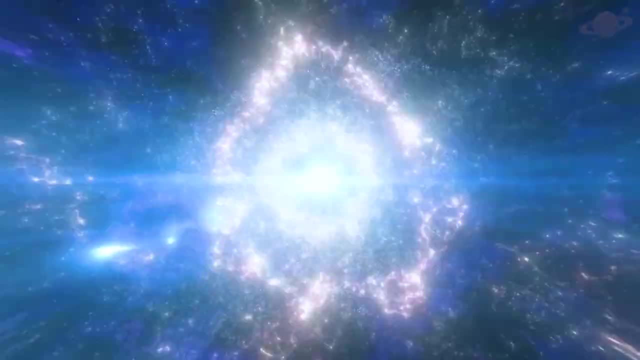 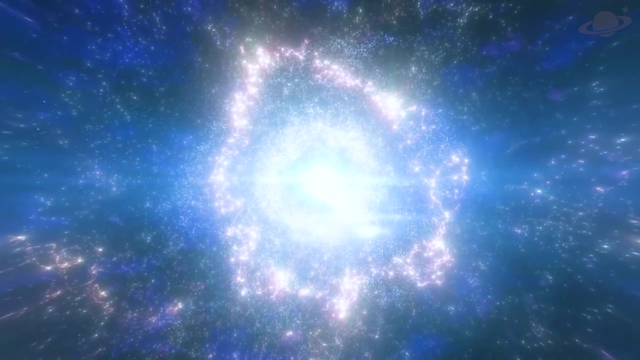 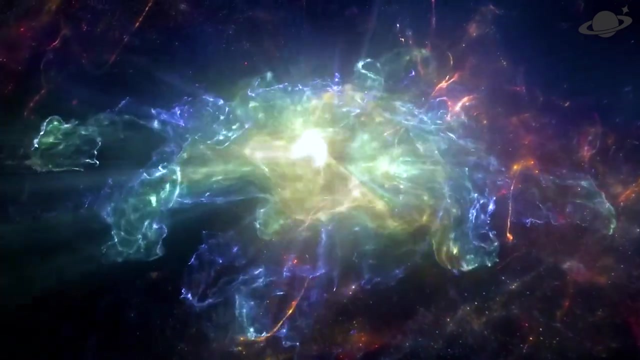 For example, if a distant galaxy were to vanish or alter suddenly due to some cosmic event linked to the universe's fate, we wouldn't become aware of it until the light from that event reaches us, potentially millions or billions of years later. How would the universe's end impact our understanding of time?